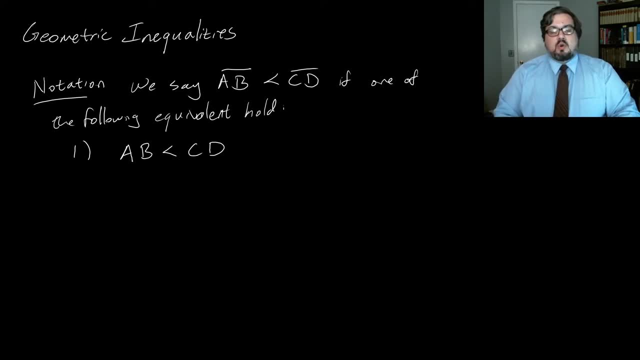 and so we're just using the normal inequality from the real numbers, but we can also express this geometrically. This is also equivalent to saying that there exists an e with e between c and d, such that the segment a- b is congruent to the segment c- e. This is how we might. 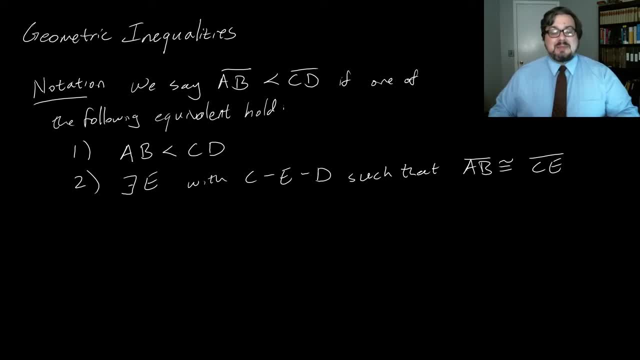 state it if we were trying not to make reference to real numbers as often. So this is a very intuitive notion. if I've got a couple of segments and I want to say that the segment a- b is smaller than the segment c- d, One way of telling that is just by looking at the distance. 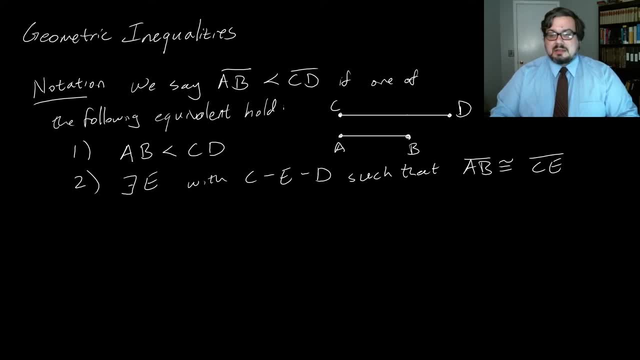 between the two. but the other way of seeing that there is that relationship between is to show that there's a point between c and d, such that the segment c- e is congruent to the segment a- b. The point is that because e is between c and d, the segment from c to 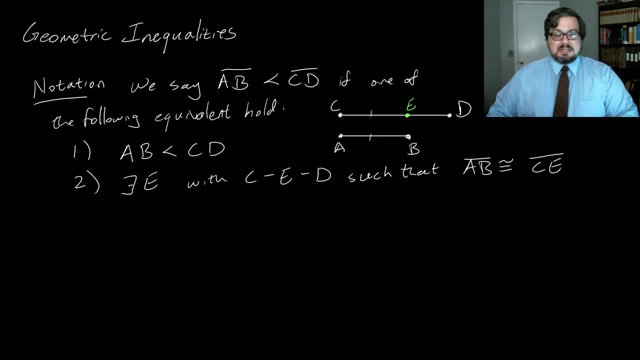 e is smaller than the whole segment a- b. Similarly, we say that the angle a, b, c is less than- and I will try to distinguish between my angle notation and my less than notation- we say that the angle a, b, c is: 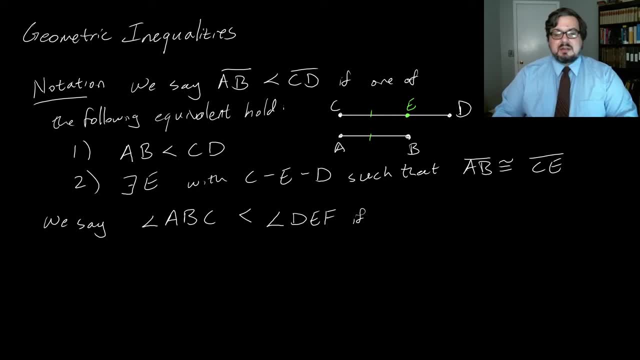 less than the angle d e f. if either- and again these are equivalent, either the measure of angle a b c is less than the measure of angle d e f, or there exists a g in the interior of angle d e f, such that the angle a b c is congruent to the angle d e g. 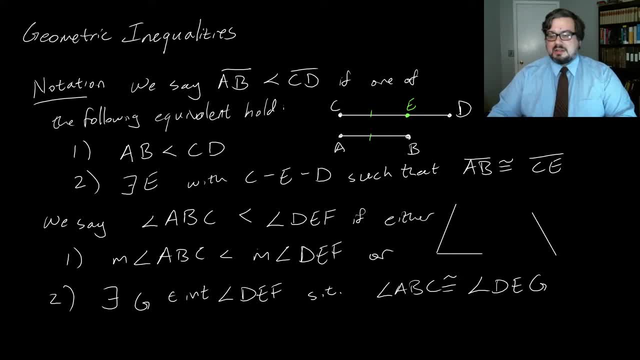 So once again, we can draw that out, We can draw a picture of what this looks like. So if I've got an angle a, b, c over here and an angle d e f, then one way of measuring that the angle a, b, c is less than the angle d e f is by saying that their measures are 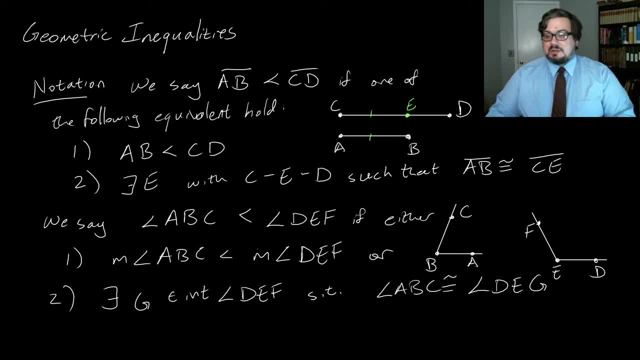 in the same relation. But the other way is to draw a picture of what this looks like. So if I've got an angle a, b, c over here and an angle d e, f, then one way of measuring that the angle d e, f is by saying that their measures are in the same relation. 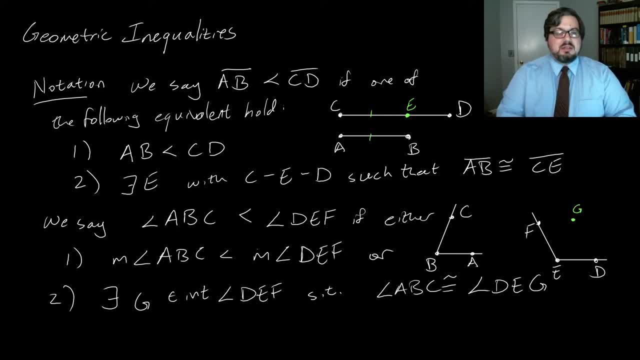 But the other way is to draw a picture of what this looks like. So if I've got an angle a, b, c over here and an angle d, e, f is by saying that their measures are in the same relation. But the other way is to draw a picture of what this looks like. 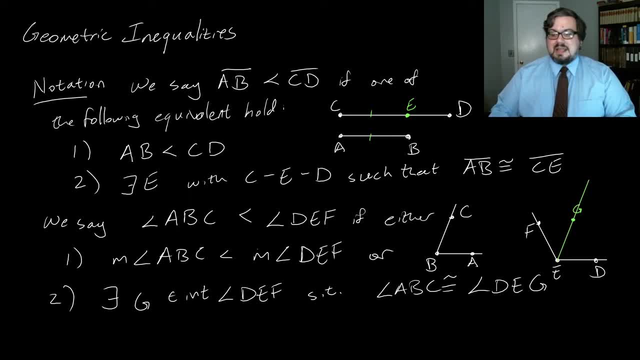 So if I've got an angle a, b, c over here and an angle d e f, is by saying that their measures are in the same relation. But the other way is to draw a picture of what this looks like. So if I've got an angle a, b, c over here and an angle d e, f is by saying that their 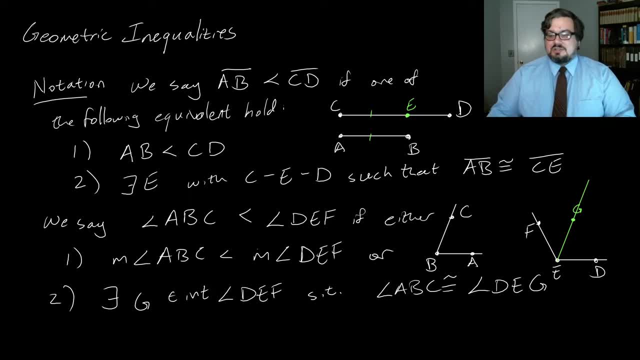 measures are in the same relation. But the other way is to draw a picture of what this looks like. So if I've got an angle a, b, c over here and an angle d, e, f is by saying that their measures are in the same relation. 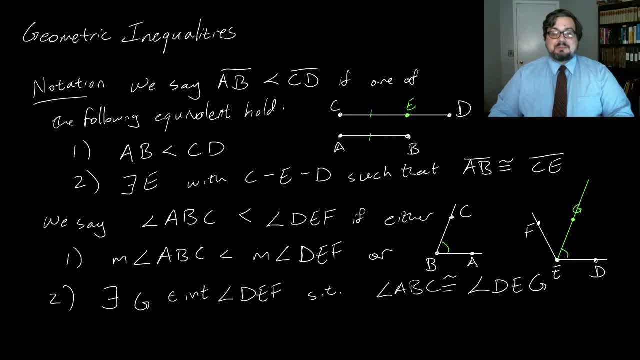 But the other way is to draw a picture of what this looks like. So if I've got an angle a, b, c over here and an angle d, e, f is by saying that their measures are in the same relation. But the other way is to draw a picture of what this looks like. 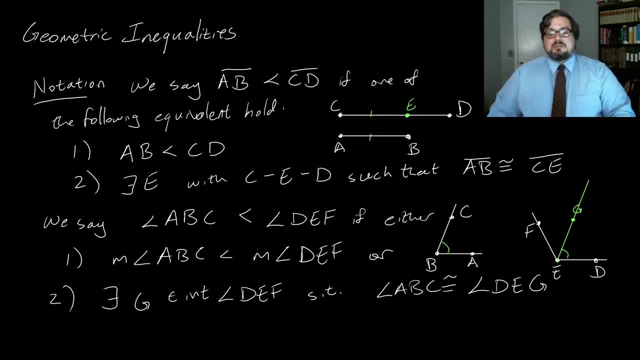 So if I've got an angle a, b, c over here and an angle d e f, is by saying that their measures are in the same relation. But the other way is to draw a picture of what this looks like. So if I've got an angle a, b, c over here and an angle d e, f is by saying that their 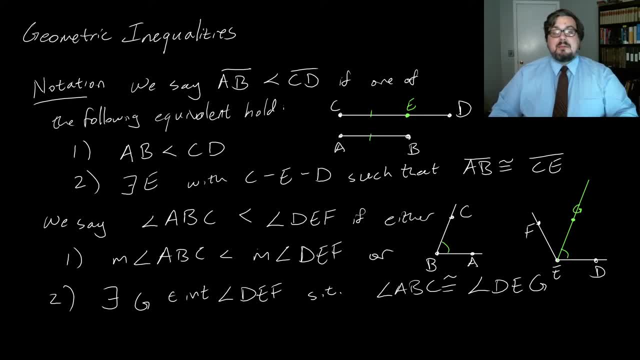 measures are in the same relation. But the other way is to draw a picture of what this looks like. So if I've got an angle a, b, c over here and an angle d, e, f is by saying that their measures are in the same relation. 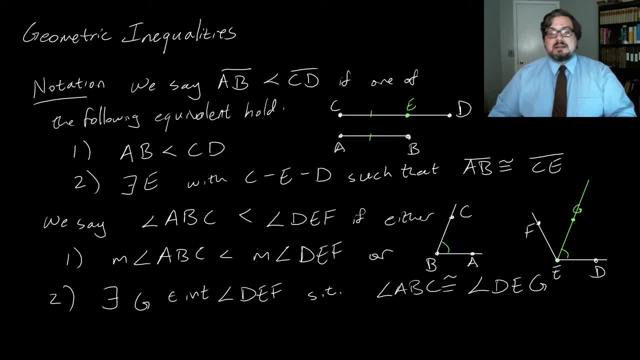 But the other way is to draw a picture of what this looks like. So if I've got an angle a, b, c over here and an angle d, e, f is by saying that their measures are in the same relation. But the other way is to draw a picture of what this looks like. 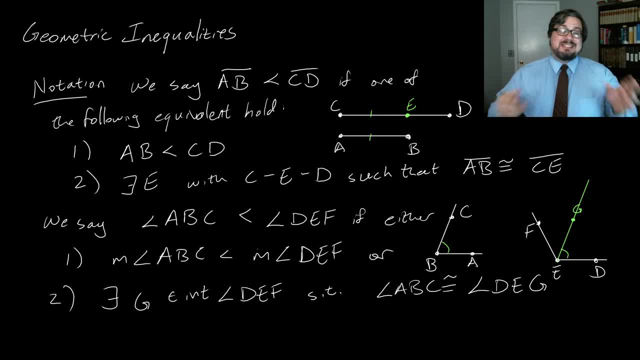 So if I've got an angle a, b, c over here and an angle d e f, is by saying that their measures are in the same relation. But the other way is to draw a picture of what this looks like. So if I've got an angle a, b, c over here and an angle d e, f is by saying that their measures are in the same relation. But the other way is to draw a picture of what's inside of the circle. So if I've got an angle a, b, c over here and an angle d, e, f is by saying that there. 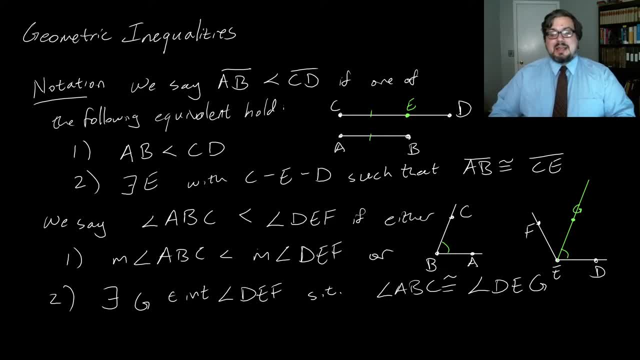 are measures in the same relation. But the other way is to draw a picture of what's inside of 1, The other way is to draw a picture of what's inside of 2.. So if the 한국계에 아버지가 이렇게 말�то 사는 besar 우선 entrepreneurship. 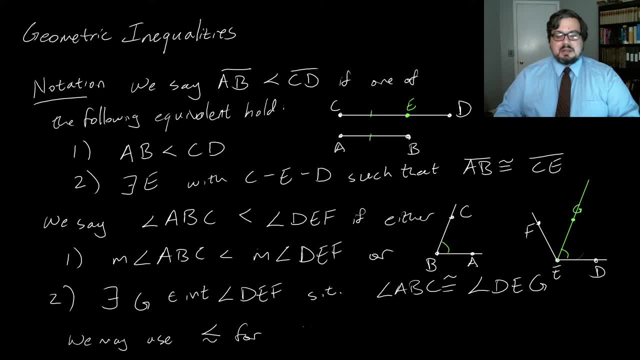 �ертв congregation에서 되어, 일하이 custom이 돌미 구성의 Haroldarios nic, Kurdistan. for less than or congruent. so in the similar way to how we use the less than or equal to notation for the real numbers, 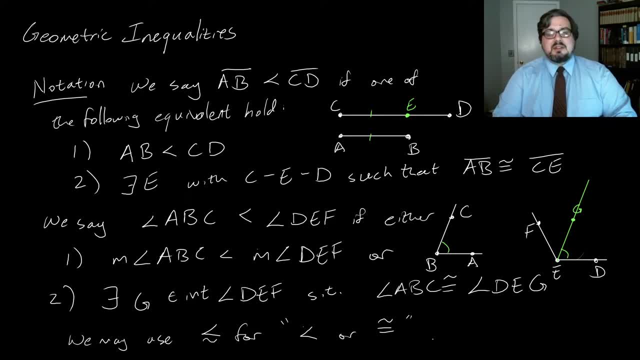 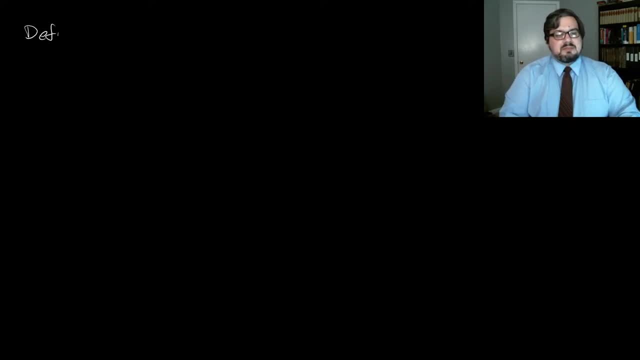 The first thing that we're going to apply these inequalities to is the notion of exterior angles to a triangle. So let's give this a proper definition. Definition 55 says let triangle ABC be a triangle and let C lie between A and D. So the picture. 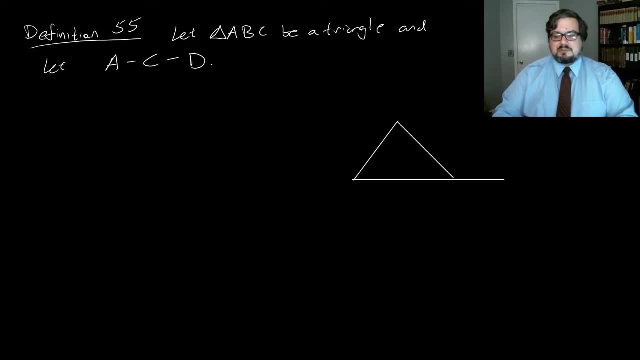 that we've got looks like the following We have: We have the points ABC on the vertices of a triangle and then a point D that lies so that C is between A and D, The angle BCD is an exterior angle of triangle. ABC and the 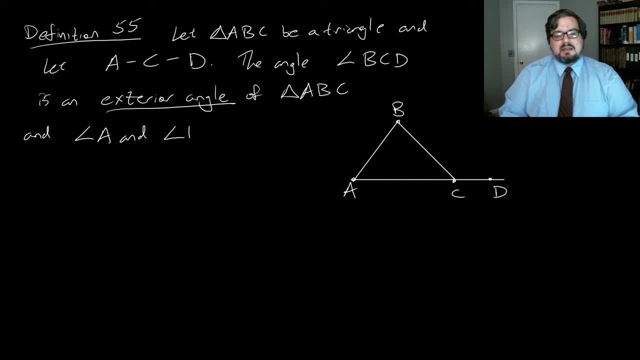 angle BCD is an exterior angle of triangle ABC. Let's use that here. Okay, Let's try to imagine the triangle ABC here. So the two angles BCD are at A and the angle at B are the Remote, or it's, I should say. 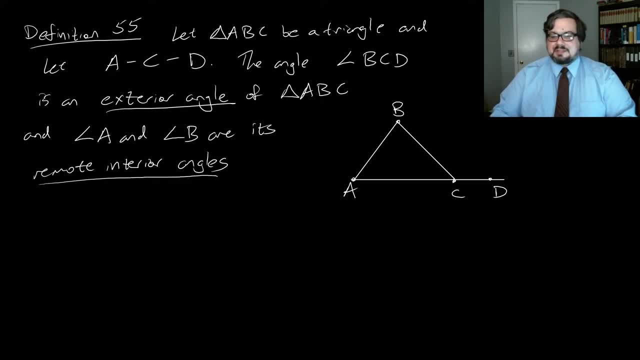 are it's Remote Interior angles? So zero angle. ABCD is the exterior, or is an exterior angle of the triangle ABC Yá, I thought it was so cool to see thatφöğ shines in my printfone Right. Congratulations, I used your optics. 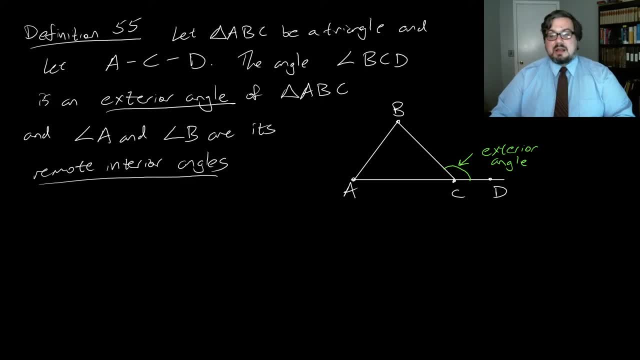 Oh, my goodness, You can see there are actually six exterior angles to a triangle, two at each vertex, And for a given exterior angle there are going to be two remote interior angles of the triangle, And these angles have a relationship that we're going to exploit very, very often. 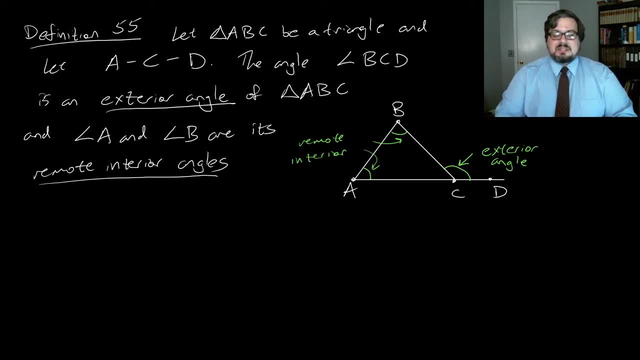 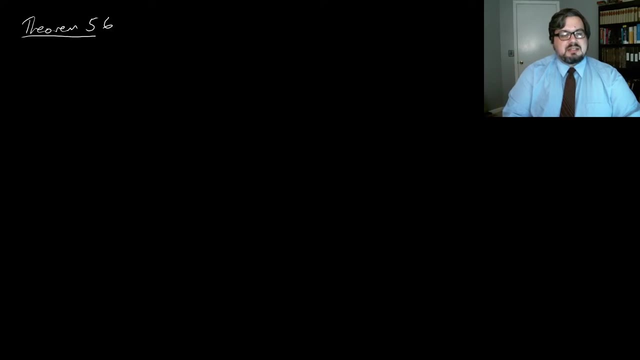 So I'm going to give myself a new page, because the proof of it will take a little bit of a statement here. So theorem 56 is called the exterior angle theorem And it says that An exterior angle theorem, An exterior angle theorem. 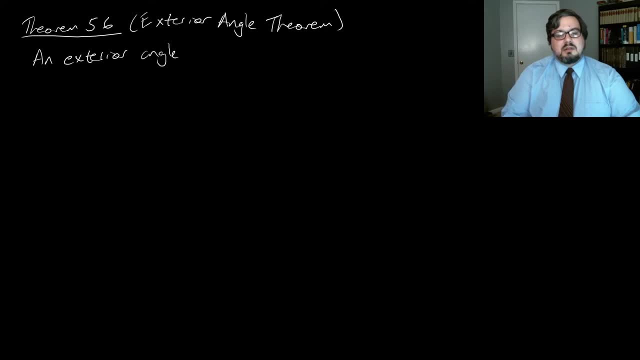 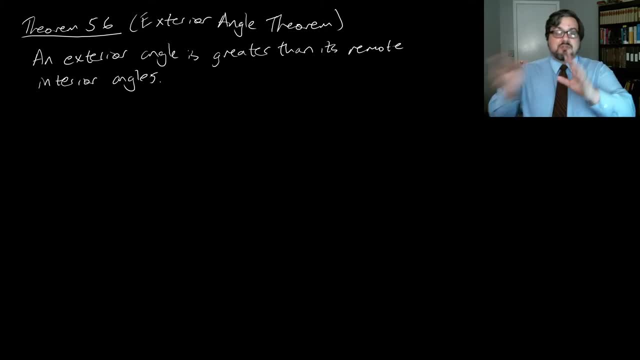 it has a greater measure, or that you can construct the smaller angle inside the larger one, which is how we're going to prove this. So let's give ourselves a similar picture to what we started with. So this is, This is, This is. 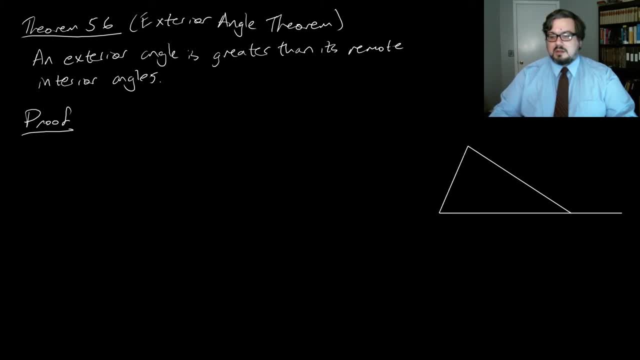 Let's see, before we start writing out the proof, let's see what we can say about this. We want to compare the angle BCD with. let's say it's going to turn out that we're going to compare it to this remote interior angle. 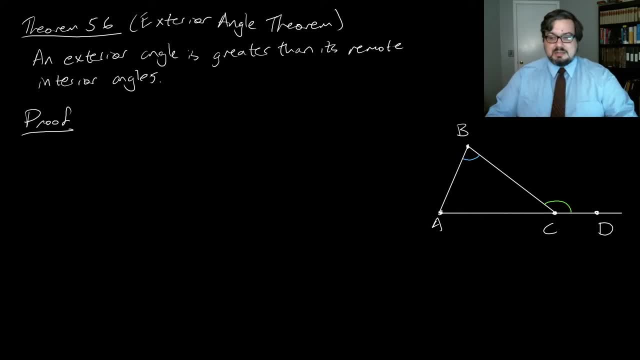 And then we're going to use facts about vertical angles in order to get the angle at A. So what we're going to try and do is construct an angle. Okay, Here in the interior of the angle BCD, which is a copy of the angle at B. 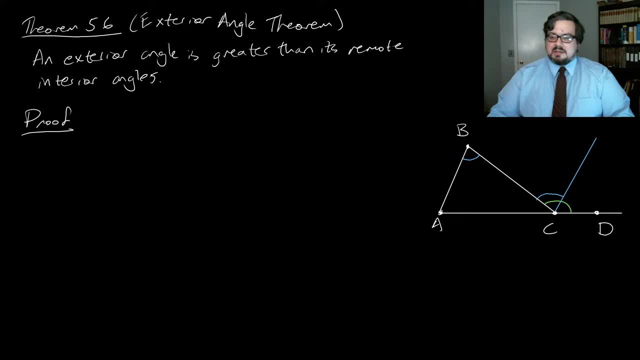 This is what we're going to try and build Now. the difficulty with doing so is making sure, of course, that if you construct this blue angle, that it actually lies within, that the blue ray lies in the interior of angle BCD. 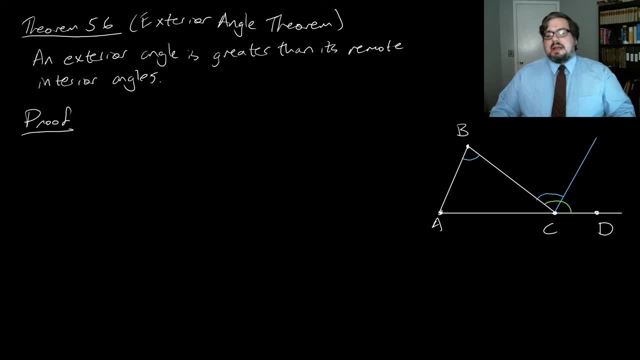 In fact, that's exactly what we're trying to prove, And so the angle- the second blue angle being congruent to the angle at B- is in fact the whole content of the proof. It's what we're trying to prove. 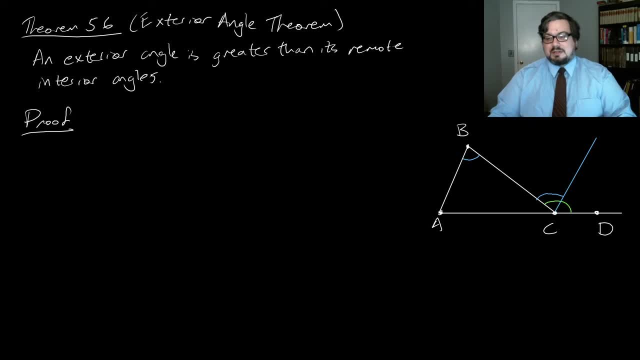 So we can't assume that we have the angle, this angle, here, blue. We're going to have to conclude. We're going to have to conclude that that angle is that the two blue angles are congruent somehow. Typically, or very often, the way that we do that is by showing that they're both angles. 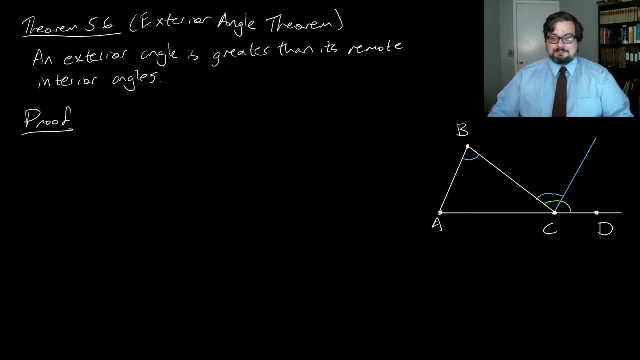 inside a pair of congruent triangles, And it's not obvious how we're going to build the build a couple of triangles that have these two angles as corresponding angles within it, but it turns out that the thing that we're going to want to do is this: 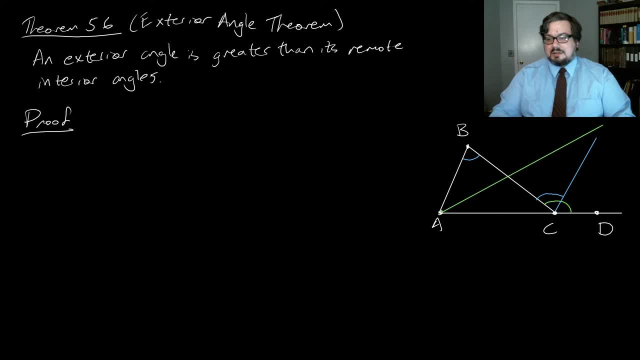 We're going to want to build a line that goes off from A like this- Let me stretch this up here- And we're going to try and show that the two new triangles we've formed are congruent to one another. Now let me give some names to these points. 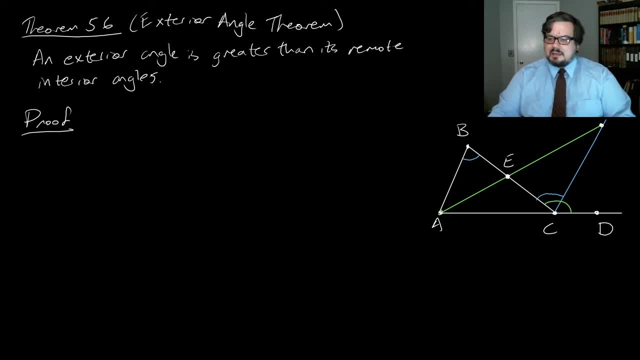 Let me call this E, Let me call this F, And it suffices to show, after we construct this- and we're going to construct it carefully to make sure we can prove this- It will suffice to show that triangle AEB is congruent to triangle FEC. 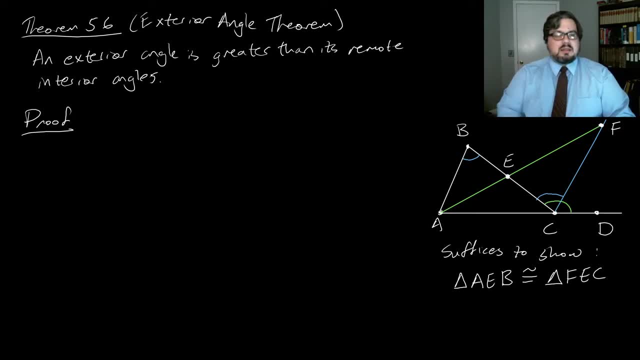 Let me actually rewrite this order to make things clearer. ABE is congruent to FCE and that F is in the interior of angle BCD. If we can show these two things, then this will show that angle ABE is congruent to angle. 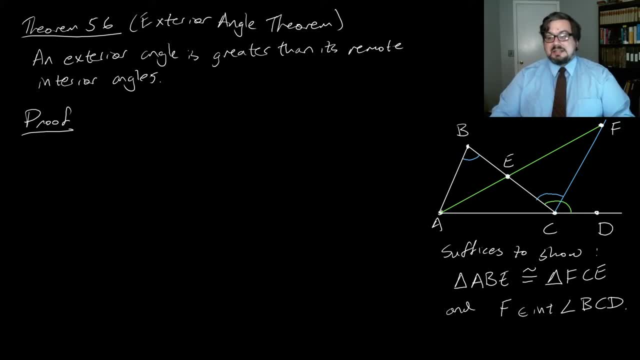 FCE and since F is in the interior of the angle BCD, that will show that the angle BCD is greater than the angle ABE. This is our goal. How are we going to conclude that these two triangles are congruent to one another? 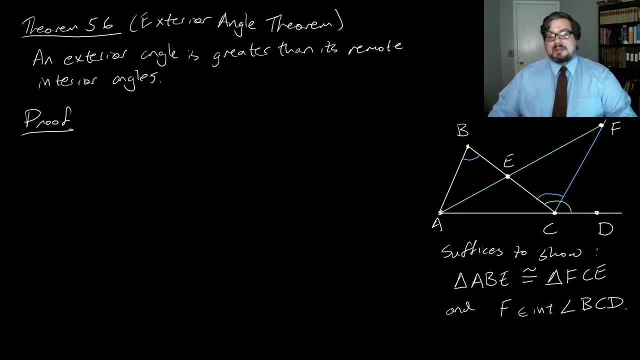 Here's where we have some problems. We have some freedom. We can basically decide where to put E and F. The first thing that we'll want to do is to make sure that the two line segments, BE and EC, are congruent to one another. 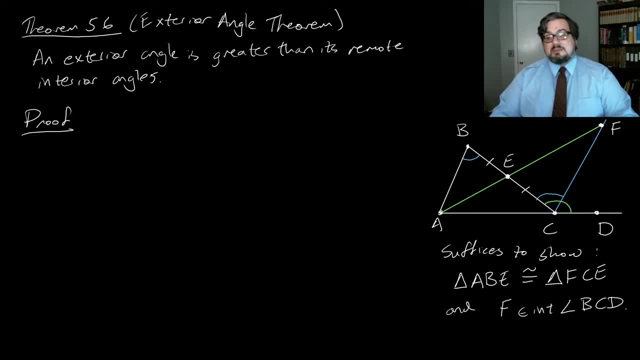 We can definitely do that. All we have to do is choose E to be the midpoint of the segment BC, and then that gives us what we want. We also, as we build this up, can ensure that the segment AE and the segment EF are congruent. 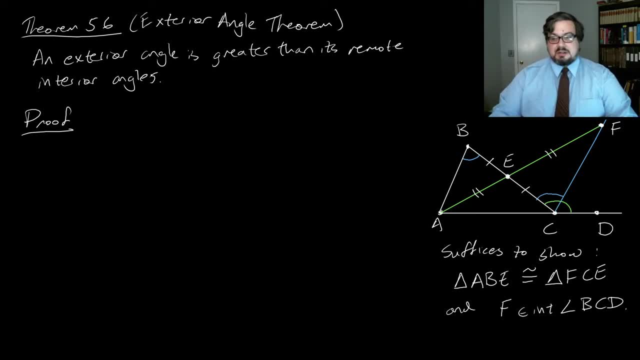 to each other. just by the segment construction theorem We can guarantee that those are congruent to each other. but now we need to either show that the segment AB is congruent to CF and use side side side. It's not at all clear how we would get at that. 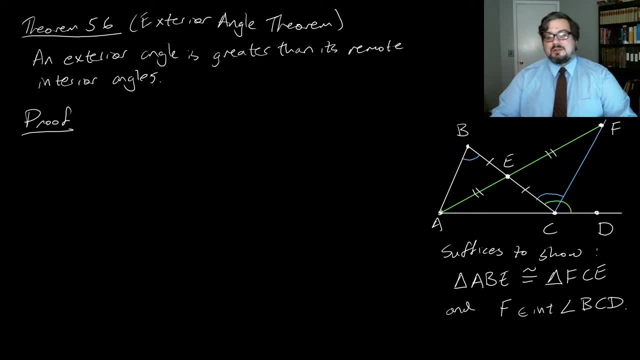 Or we need to show that the angle in between the sides marked 1 and 2 are congruent in these two triangles. Well, here's where we can use the fact that we know that vertical angles are congruent to each other. So once we construct E and F properly, we will be able to show that the triangle ABE is congruent to the triangle FCE by side-angle-side, which will give us the congruence of the blue angles, which is what we were going for. 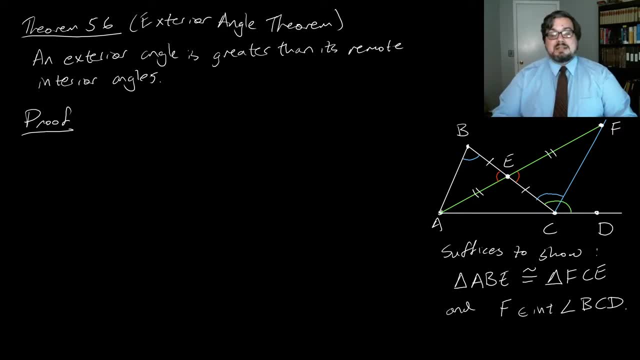 So there's the idea. Let's write down the proof. So we could say: first of all, notice, the theorem doesn't give us any notation here. So all the notation that we did with setting up the triangle and everything we need to specify in the proof. 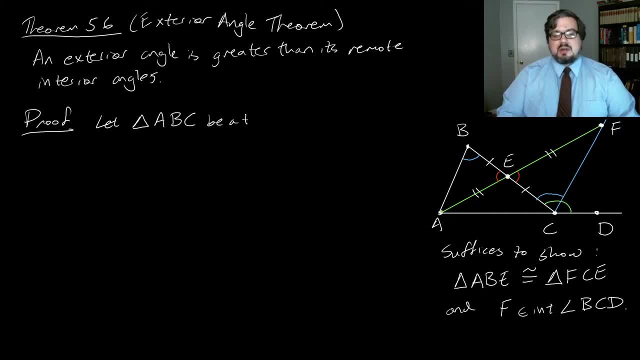 So we need to say: let triangle ABC be a triangle and let A to C to D. So we're introducing the point D and we say that it satisfies the condition ACD, And so we're considering the exterior angle BCD. 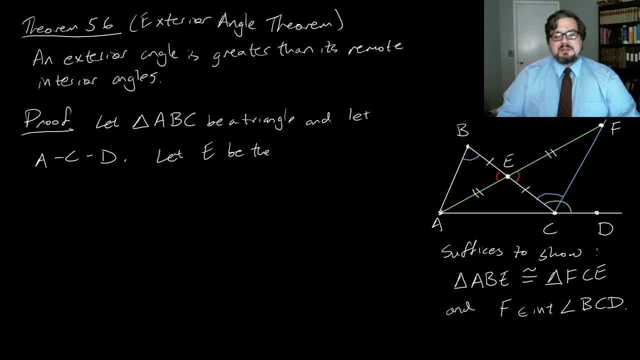 Now we can let E be the midpoint of the segment BC. We've shown that every segment has a midpoint. This is okay. And we can let F be in the ray AE, such that the segment EF is congruent to the segment AE by the segment construction theorem. 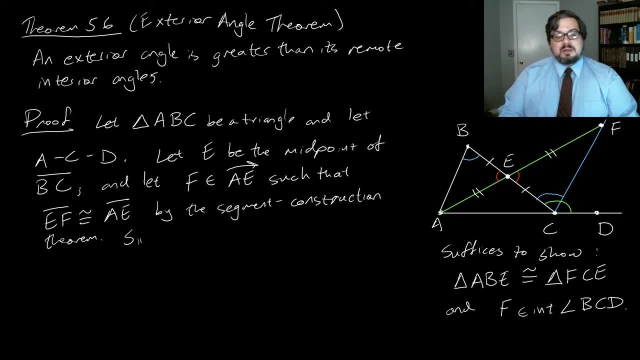 So now we have that, since the segment BE is congruent to the segment CE by construction, the angle BEA is congruent to the angle CEF, since they are vertical angles, Okay, And segment AE is congruent to segment FE. 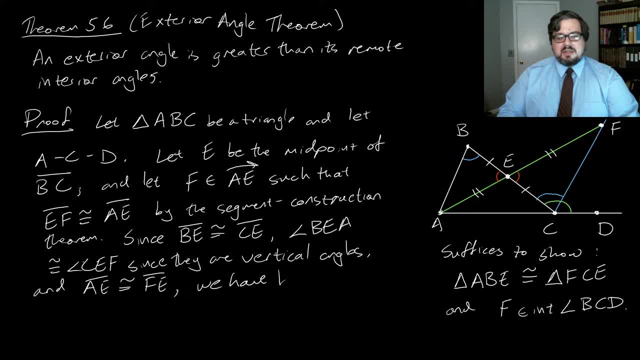 We have that the triangle ABE is congruent to the triangle FCE, where the triangle ABC is congruent to the triangle EF, Okay, And we have that the triangle AE is congruent to the triangle FCE by construction, since they are vertical angles. 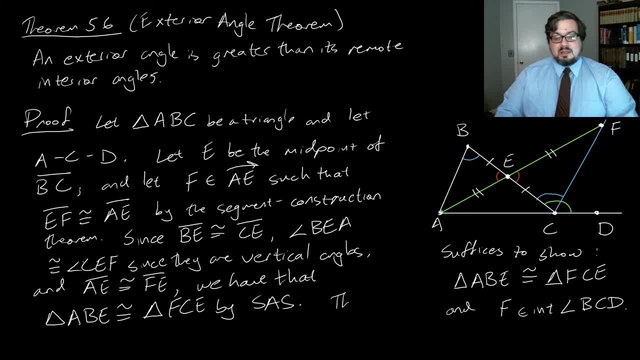 Okay, side, angle side. Now that gives us the congruence that we need, but we also need to know that F lies in the interior of angle BCD for this to work. Well, we actually proved this as a theorem By: 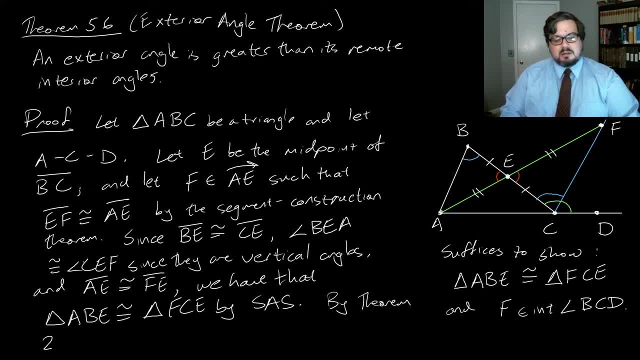 theorem 29, F is in the interior of angle BCD. Thus angle BCD is greater than angle ABE. So that gives us the relationship that we're looking for for the angle BCD. So that gives us the relationship that we're looking for for. 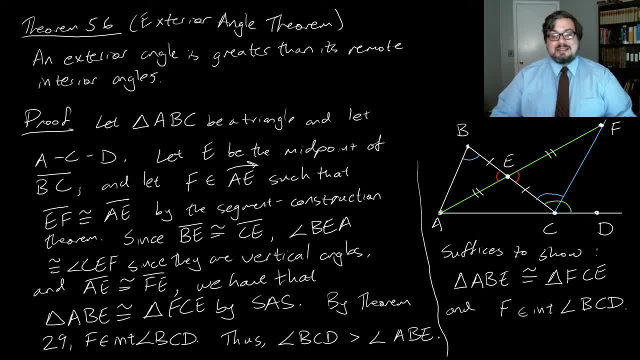 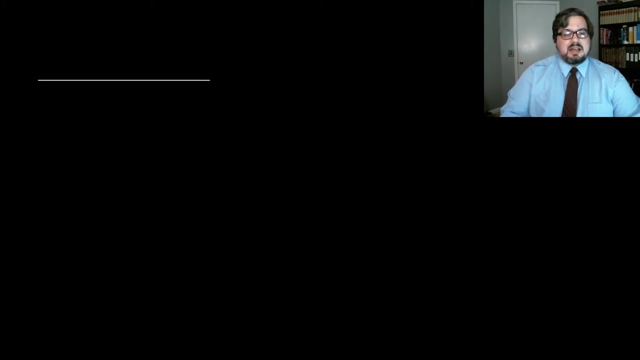 the exterior angle BCD, and the remote interior angle at B. Alright, so let's talk about how we get that the angle at BCD is greater than the angle at A in the original triangle. So let's get our same diagram again, but with we don't need all of the pieces that we had before. We've 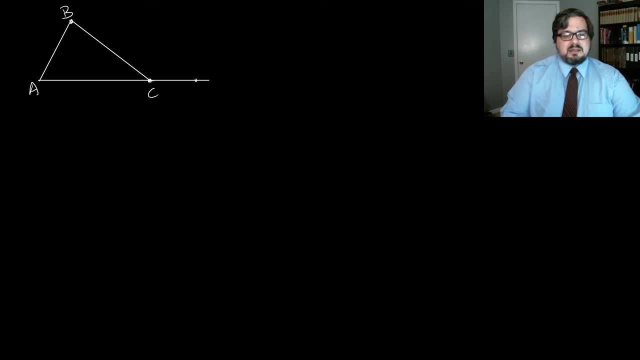 got A, B, C, D and we've shown that the angle BCD is greater than the angle at B. So now we want to show that it's greater than the angle at A. Well now, let's let G 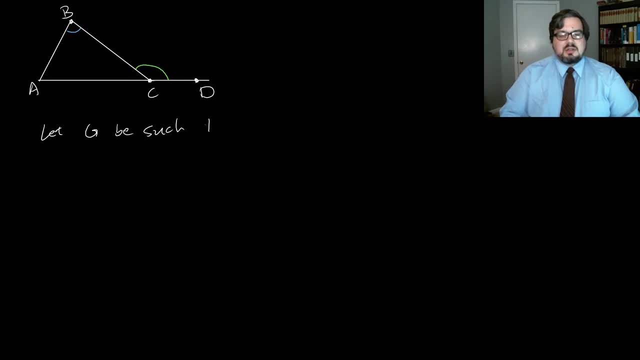 be such that B, C, G- We're actually going to get at this conclusion by looking at another exterior angle. So we're going to look at the sorry. we are going to look at the exterior angle. So we're going to look at the three Novits and that hexagonal angle And we're going to get the 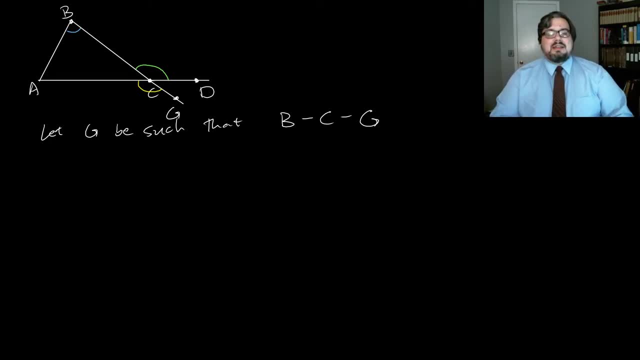 angle here, the yellow angle. The yellow angle is also an exterior angle of the triangle. But but now if we run the same argument through with this angle that we did for the green one, fr" eq, M, b inx. 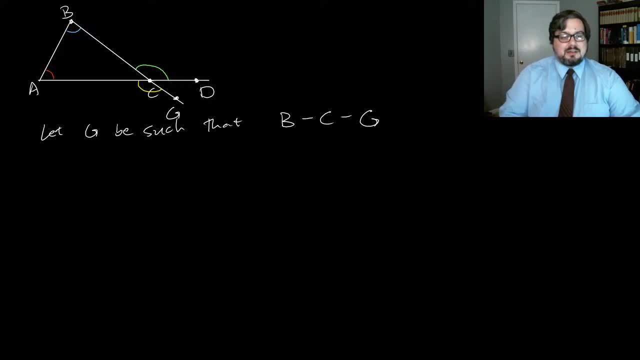 h in x" Н greater than the angle at A. So a similar argument with A and B switched and G replacing D shows that shows that the angle ACG is greater than the angle at A. Well, now we can note that since the angle ACG is greater than the angle at A, the angle ACG is greater than. 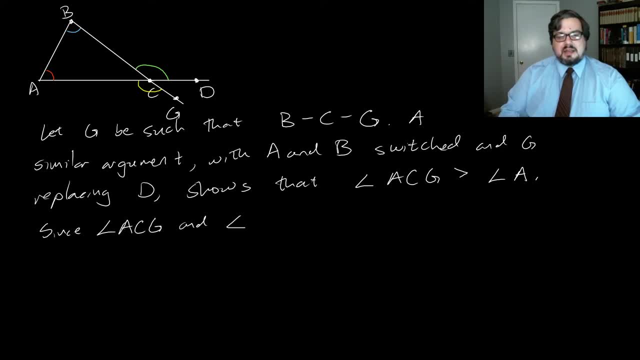 the angle ACG and the angle BCD are vertical angles. Angle ACG is congruent to angle BCD. Thus, angle BCD is congruent to angle ACG, which is greater than the angle at A, And while we haven't explicitly defined the angle ACG, we can say that the angle ACG is greater than the angle. 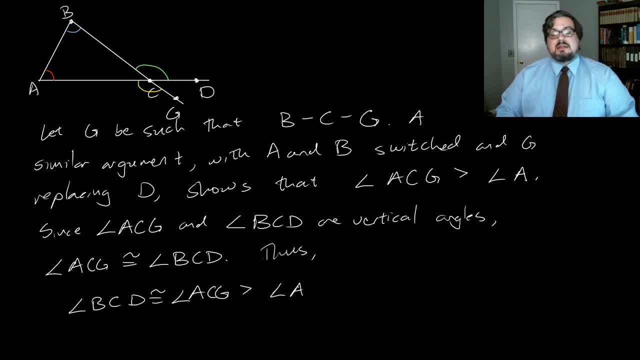 BCD is greater than the angle ACG. So, if we have explicitly written this out, it is true that congruences and inequalities of geometric objects chain together in the same way that they do for numbers, because in fact they are just statements about real numbers And 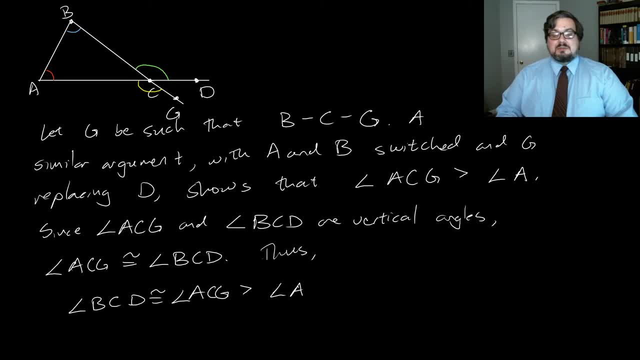 so, in particular, since angle BCD is congruent to angle ACG and angle ACG is greater than angle A, our conclusion is that angle BCD is greater than angle A. Rotation at score is still the same as range X, so angle ACG can beаем worship of both terms. 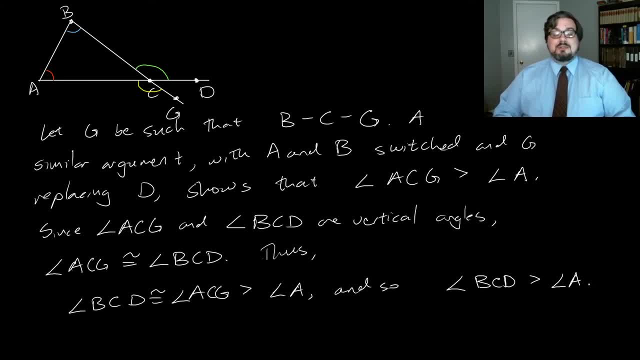 Of course right angle BCD remains incorrect for first energies. So here long approach to QD refers to angle finished at a vector. So we get that the angle BCD, the exterior angle, is greater than either of its remote interior angles. 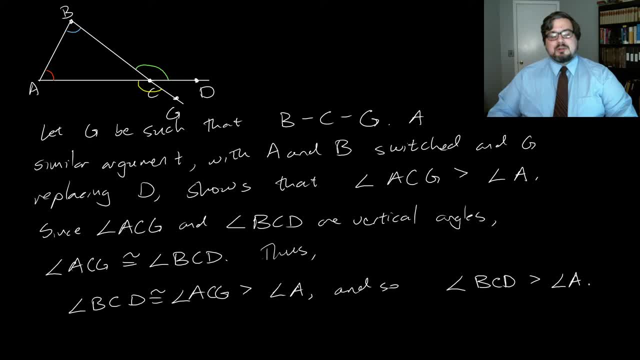 This turns out to be quite useful. Now you may be thinking to yourself. You may remember that in high school geometry you are often told that the measure of the exterior angle is exactly equal to the sum of the make built surface linear vectors. This is amazing. They are very, very nice numbers. 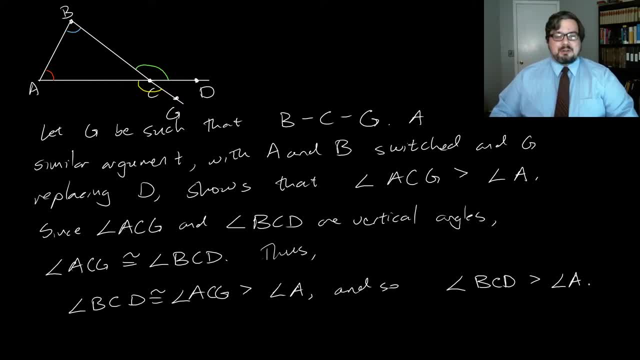 Let me explain in a little bit. So long approach to QD refers to the measurement of the exterior vector, which is equal to the sum of the make built surface linear vectors. which is equal to the make built surface linear vectors, the measures of the remote interior angles. This is, however, not always true. It is true. 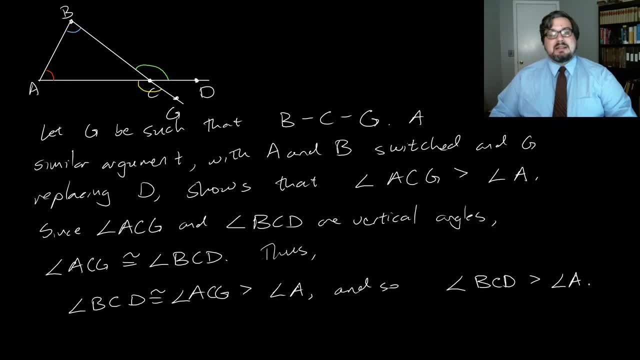 in some geometries, including the familiar Euclidean geometries that you learn about in high school, and in other places. However, there are some geometries where that isn't necessarily the case. We're going to be talking more about this soon, So for now, 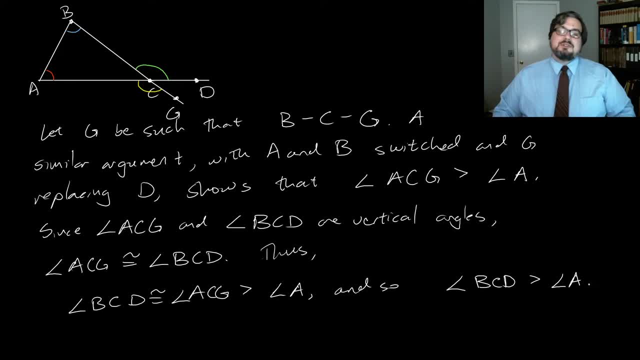 all we can conclude is that the exterior angles are always greater than any one of the remote interior angles of that triangle. This result on exterior angles has a surprising power. We are going to use it over and, over and over again in order to prove all sorts of things. 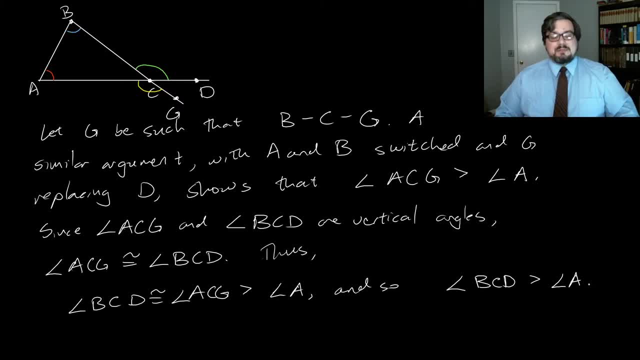 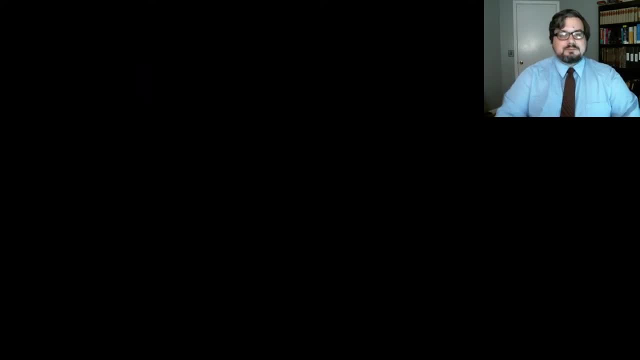 about geometric optimization, As if we had an absolutely perfect grid of objects that, on the face of it, don't have anything to do with triangles at all. For instance, let's consider the following: Let's consider corollary 57,, which is really the second half, or the uniqueness part, of a theorem. 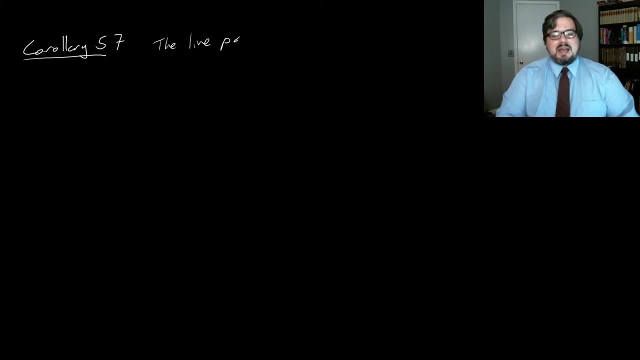 that we stated before. Corollary 57 says the line passing through point P and perpendicular to a line not containing P is unique. So this is the uniqueness part of the statement we had before which said that, given a line and a point and 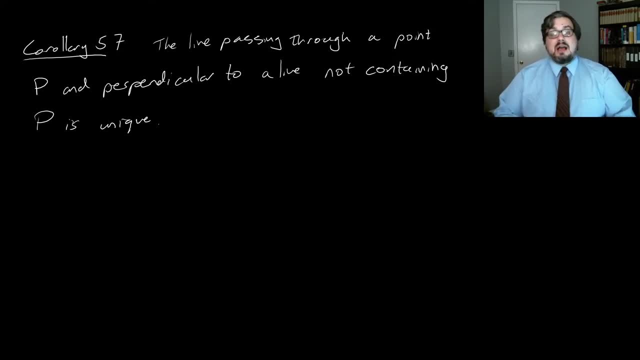 a plane containing them, there is a unique line that is perpendicular to the first line that passes through the point P, And what this is telling us is that, in the case of that theorem, where the point P does not lie on the line that there is a unique line, 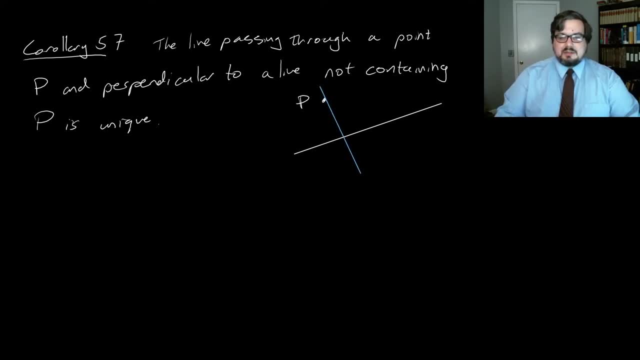 passing through P that is perpendicular. Now, quite often, the way to prove that there's a unique one of something is to assume that there are two different ones, and either prove that they have to be the same or prove that you arrive at a contradiction by making this. 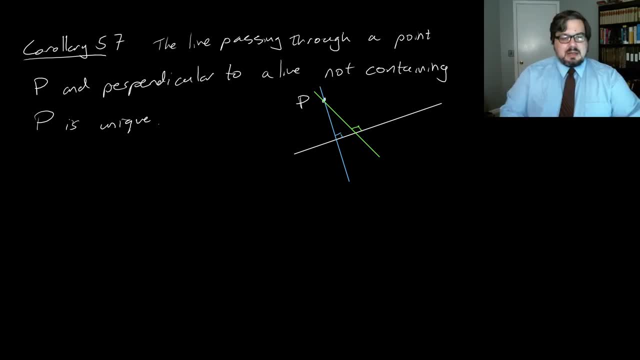 happen. So let's go, Let's go to a proof. Let's let L be a line, P a point, not on L, and let L prime, L, double prime, be lines, be two lines containing P and perpendicular to L. So that's this statement that I've got right here. So when 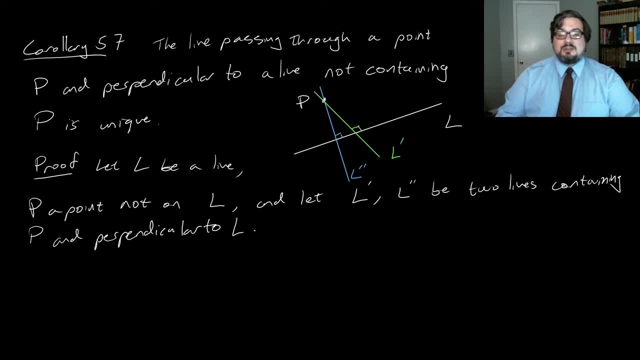 that happens, then, because L prime and L double prime are perpendicular to L, they must share a point with L. So let's let Q, Let Q be the point in L prime intersect L, So that'll be this point right here, And 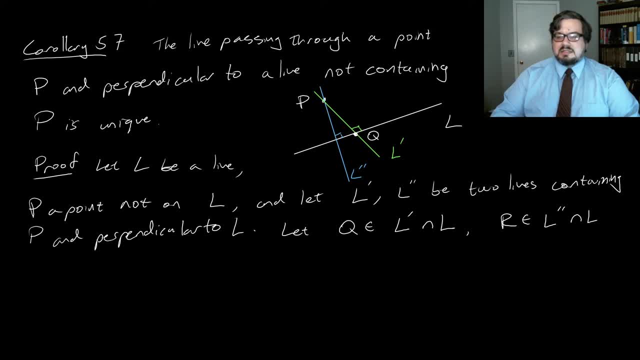 let's let R be the point. in L double prime intersect L. Since L prime is not equal to L double prime, we've assumed that they are two lines, that there's two different lines, Since L prime is not contained in L double prime, but both. 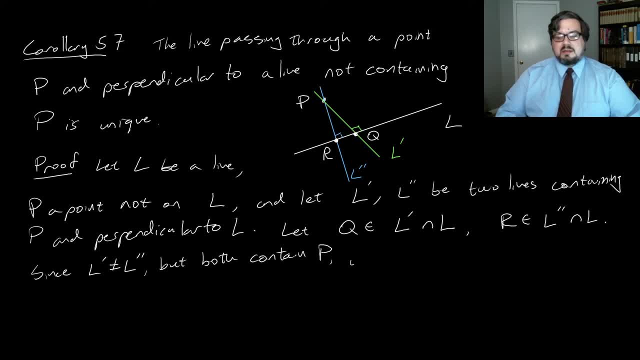 contain P, we have that Q is not equal to R. If L and L prime contained the same point, if Q and R were the same and they also contain P, then in fact they would be the same line. We've assumed that there are two of them. 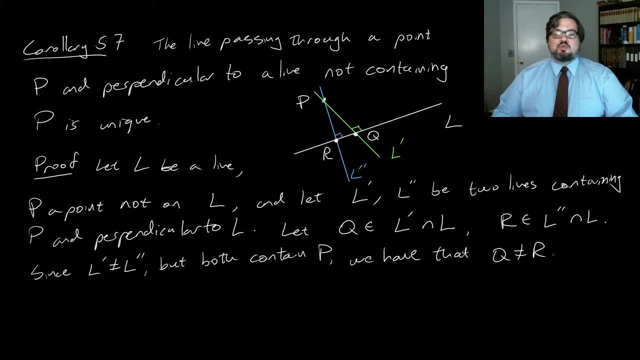 But now you'll notice that we've created a triangle from P to R to Q, And we can use the exterior angle theorem to show that this situation we've described cannot happen. Now, to do that, let's let T be such that R goes to Q goes to T. So let's say that: 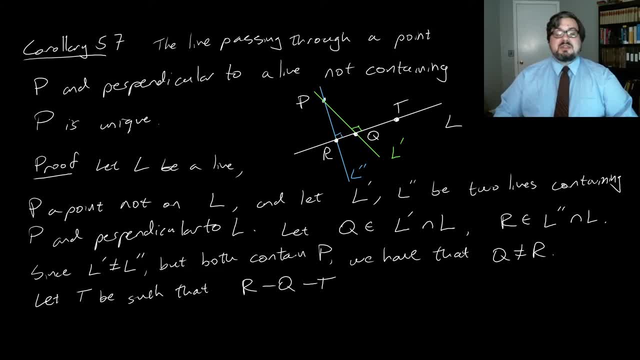 we give ourselves a T over here, and the only reason we're choosing a T here is so that we can talk about angles. Now we have that the angle PQT is exterior to the triangle PRQ, and so we have that angle PQT has to be greater than either of its remote. 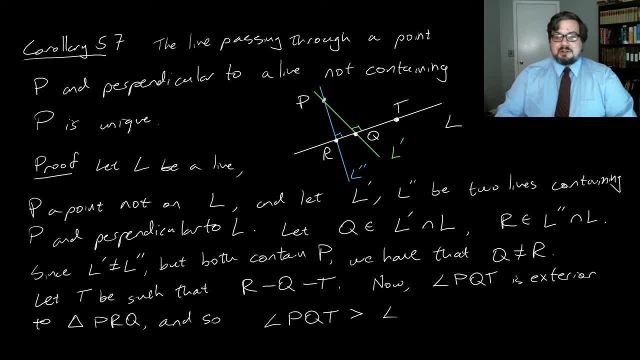 interior angles. One of its remote interior angles is the angle at r, so this is greater than the angle PRQ. However, this is a contradiction. Our assumption was that L prime and L double prime were both perpendicular to L, which means that any angles formed between them. 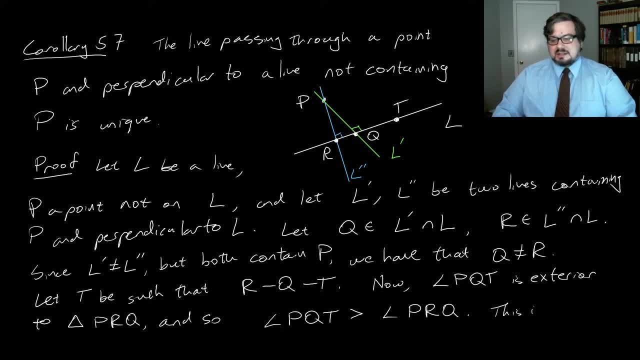 are all right angles, so this is a contradiction. since they are both right angles, Therefore they are congruent and, in particular, neither one is greater than the other. A lot of the problems and theorems that we're going to be looking at are usually congruent. 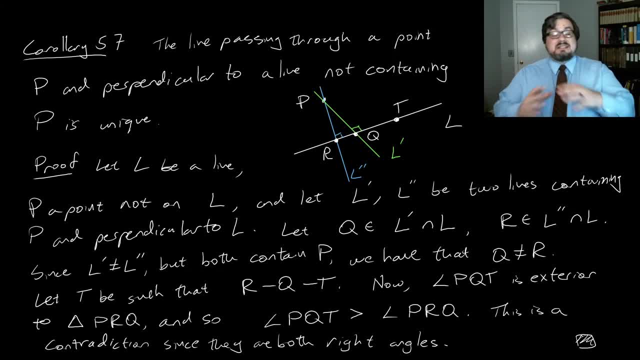 However, because of the fact that they are all right angles, they are all Cu squared- going to be able to be solved by essentially sketching out the situation we're trying to prove doesn't happen, and then show that something about what we've 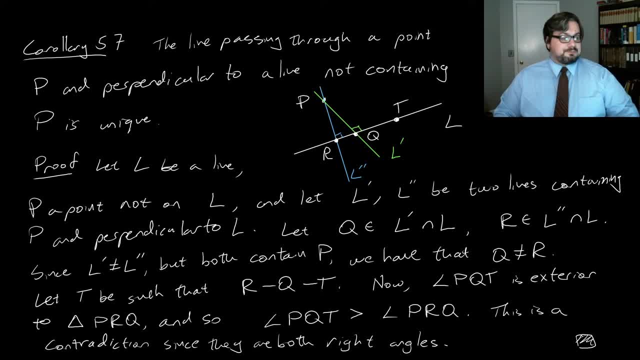 drawn has violated the exterior angle theorem. The exterior angle theorem is also very useful for proving the following result, which is sort of an expansion upon the isosceles triangle theorem. So the isosceles triangle theorem said that if you've got a triangle and two sides are congruent, then 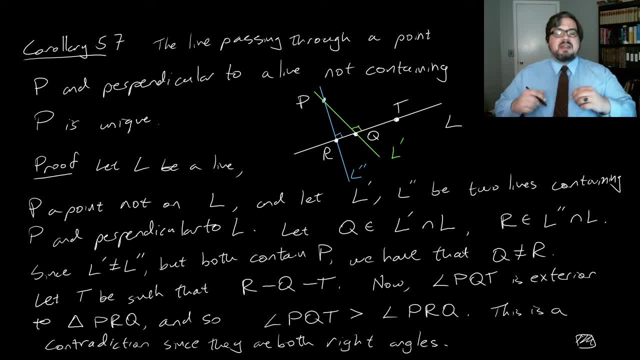 the angles opposite them are congruent, But it didn't say anything about what happens if the two sides were different, of course. And if the two sides are not congruent, well, one of them has to be greater than the other under our new 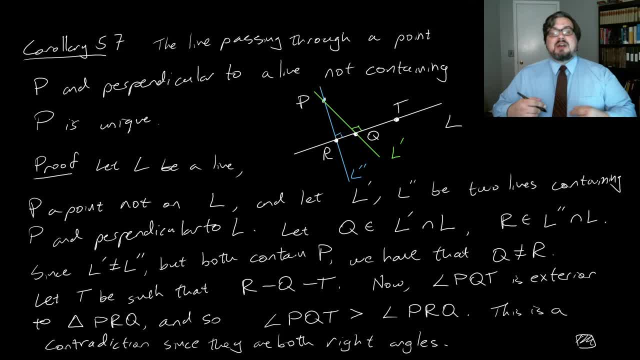 notation. And if you look at the angles opposite them, they can't be the same either by the corollary, the converse direction of the isosceles triangle theorem, And so one of them has to be greater than the other And, as it turns out, the larger 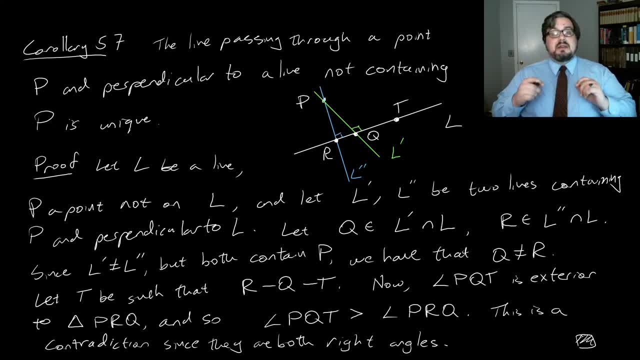 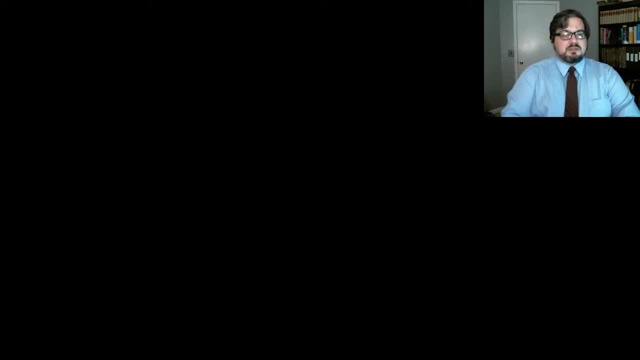 sides have to be opposite the larger angles, and this is a very useful fact that we're going to be able to take advantage of many times. So let's look at theorem 58, which says that if triangle ABC is a triangle, then—we'll say this efficiently—segment AB is greater than segment AC if and only 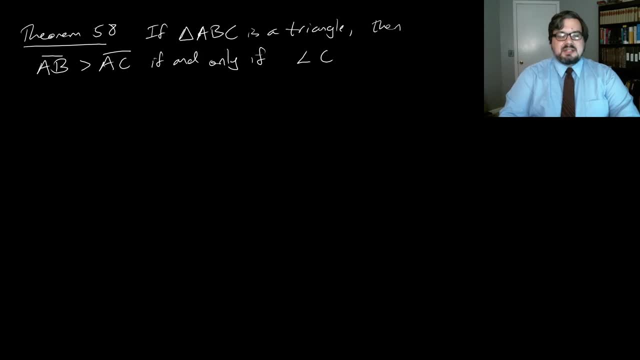 if the angle C is greater than the angle B, get a sketch of what's going on. so we've got a B, C and we want to talk about what happens when these various angles and segments are are greater than each other. so let's go to. 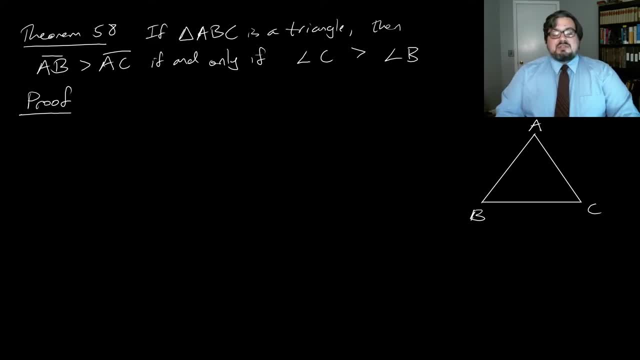 the proof. we want an if, and only if. so we're going to. we're going to do this in a slight variation from the standard way of doing things. usually, when you prove an if, and only if, you assume the first statement, prove the second, then assume the second statement, prove the. 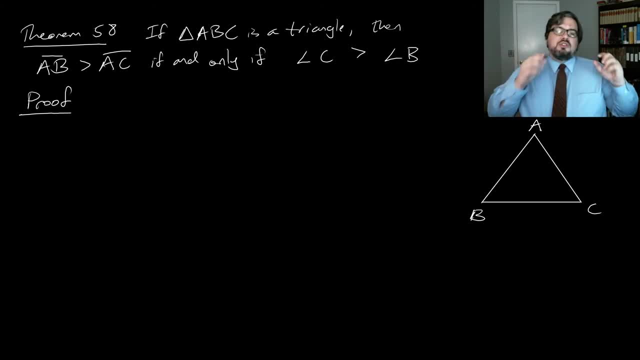 first. an alternative version is the following: you assume the first statement is true and prove the second. the first part stays the same, but then you prove that if the first statement is false, then the second statement also has to be false. this is basically taking the contrapositive of. 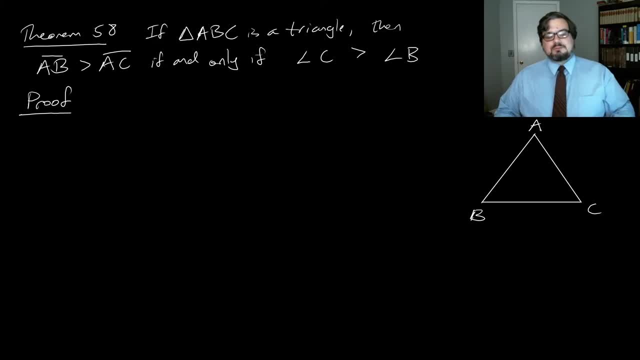 the right to left direction, so it's completely logically equivalent, but sometimes easier. the first part, as I said, though, goes the same, so let's suppose that segment a b is greater than the segment a c. so what that means is that? what several things that it means, but what one of the things it is is the following: we can let 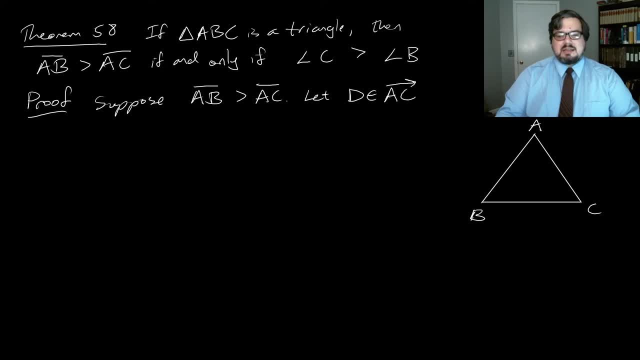 D be in the ray a C, such that the segment AD is congruent to the segment AB, which implies that C will lie between A and D. So we're assuming that the segment AB is greater than the segment AC, which means that we will be able to find another point D over here with the property. 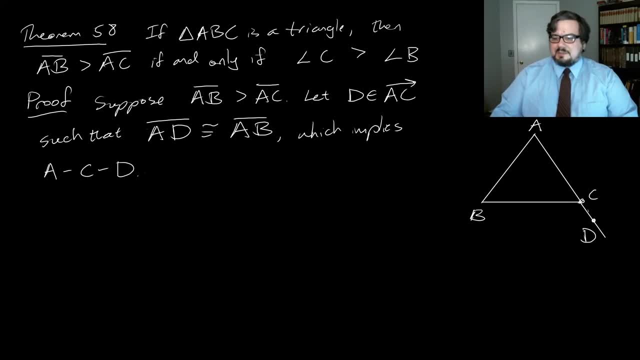 that the segment AD. I'm going to add a single tick mark to indicate that it's congruent to the segment AB. Well now, that means that triangle ABD is isosceles. Now, triangle ABD is isosceles. 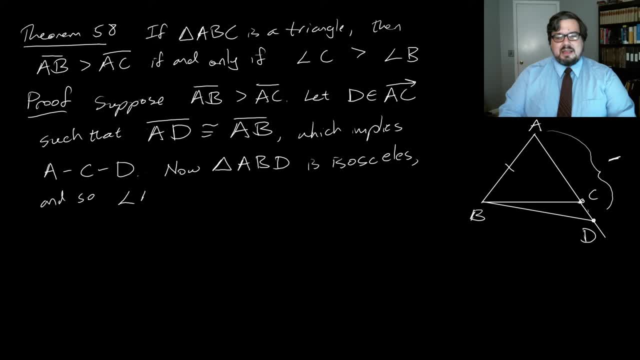 And so that means that the angle ABD is congruent to the angle ADB. So we have that the two blue angles are congruent to one another. Now, they don't look congruent to one another here because I've, because the way that I've sketched things out, 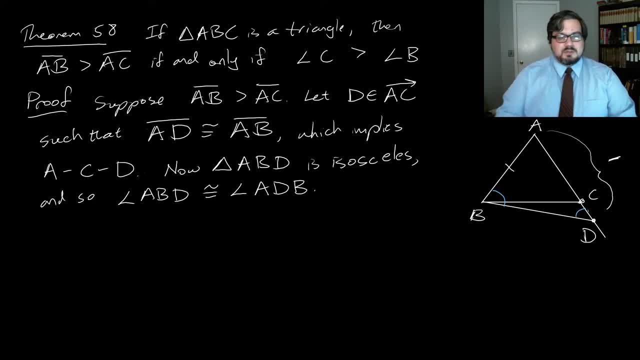 But remember, the sketch isn't the proof anyway, So we're just using it to keep track of our work. Excuse me, So now we want to look at a couple of things. So First of all, the angle ACB is an exterior angle to the triangle BCD. 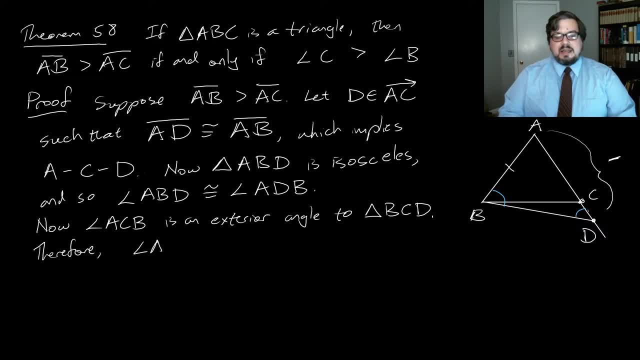 Therefore, the angle ACB, which is the angle that we're looking for in the first place, has to be greater than the angle CDB, which, of course, is the same as the angle ADB. So that is same andulatoric angle. 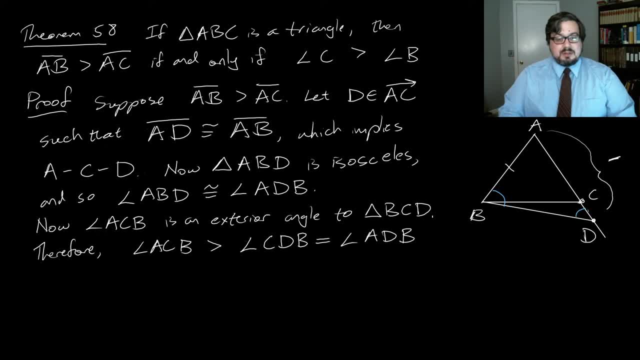 But that is congruent to this angle, Which itself is congruent to the angle ABD. So we've shown that the angle ACB is greater than the angle ADB, so which is congruent to the angle ABD. So green is greater than blue here. 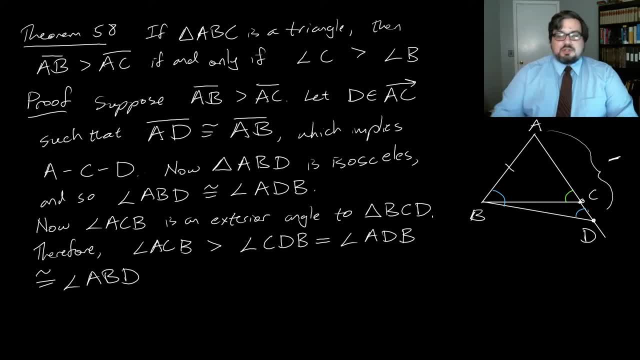 We're not quite done yet We cause. we want to show that the green angle is greater red angle ABC, and we have that it's greater than the angle ABD. However, we're nearly done here, Since C is in the interior of segment AD. 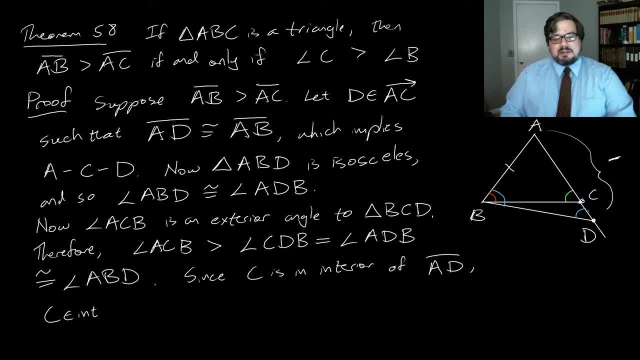 C is in the interior of angle ABD and so, by definition of inequalities of angles, we have that angle ABD is greater than angle ABC. So we have that ACB is greater than CDB, which is equal to ADB, which is congruent. 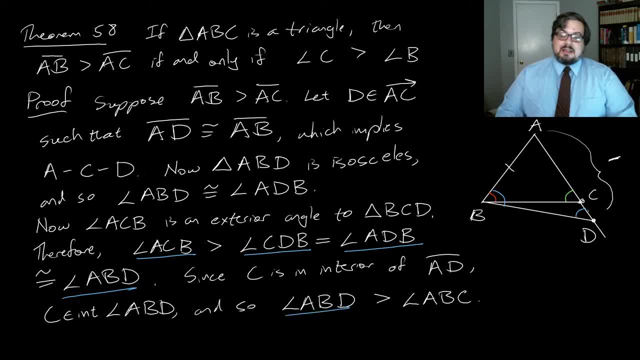 It's congruent to angle ABD and we have that angle ABD is greater than angle ABC. So that means at the end of the day, angle ACB is greater than angle ABC, which is what we wanted to prove here. So that gives us the forward direction that if segment AB is greater than the segment AC, 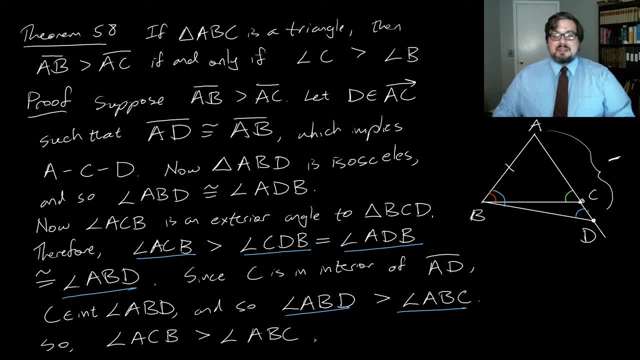 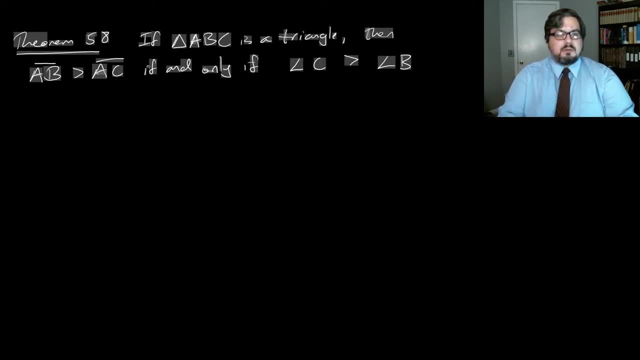 then the angle at C is greater, Then the angle at B. So that's half the proof done. Let's do the other direction. So now we're going to prove the other direction, But, as I said, instead of assuming that angle C is greater than angle B. 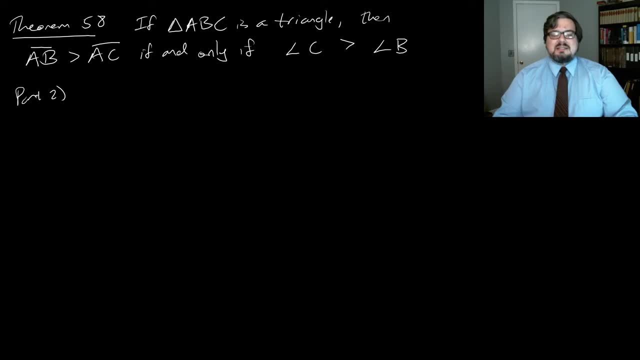 which winds up being not true and not nearly as easy to work with. we're going to assume that the segment AB is not greater than the segment AC. So now suppose that the segment AB is not greater than the segment AC And we're going to try to prove that the angle C is not greater than the angle B. 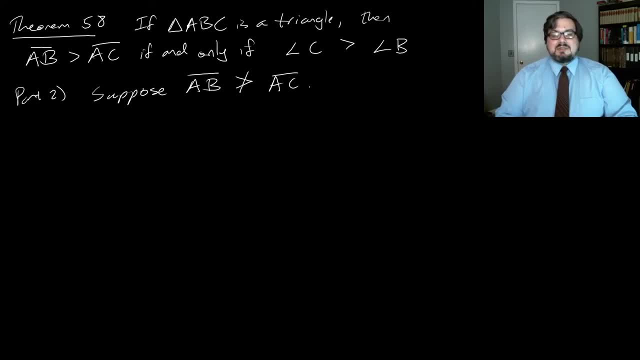 So it, the segment AB is not greater than the segment AC. That means that either the two segments are congruent or the segment AB is less than the segment AC. Now, if the segment AB is congruent to the segment AC, Then by the isosceles triangle theorem we have that the angle C is congruent to the angle B. 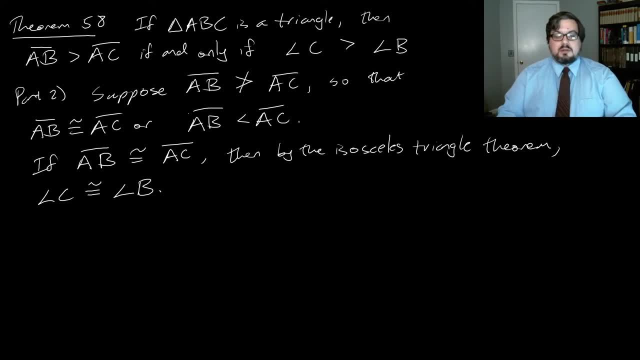 On the other hand, if the segment AB is less than the segment AC, then by the first part of the argument we already proved that if one segment is greater than another in the triangle, then the opposite angles have the same value. They have the same relationship. 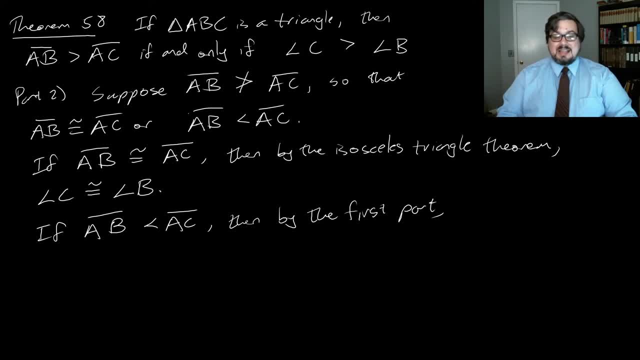 So that means that if segment AB is less than segment AB, then by the first part we have that angle C. the angle opposite, the segment AB, is less than the angle at B. So that means that in either case the angle C is not greater than the angle B. 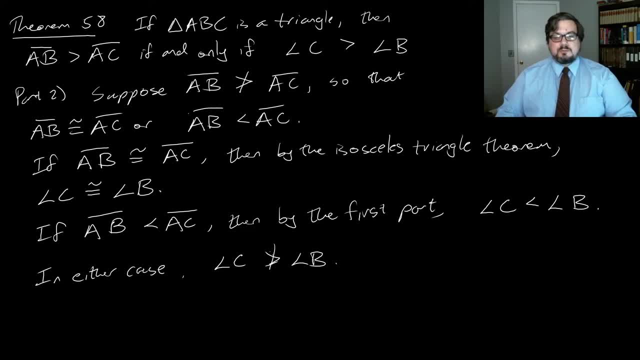 which in그렇able. So that means that if the segment AB is not greater than the segment AC, then the segment C is not greater than the segment B a 1. So we proved that if the segment AB is greater, then the angle C is greater. 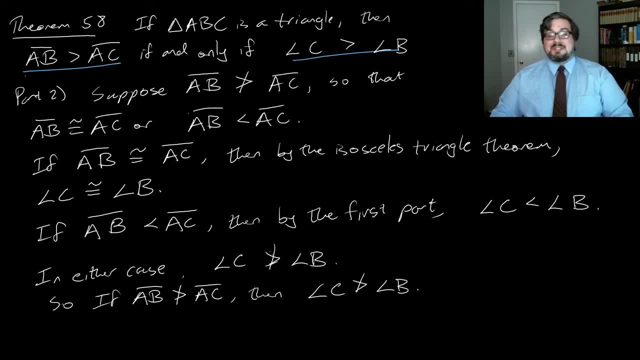 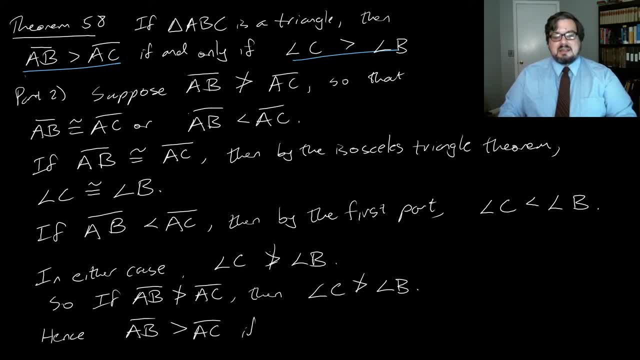 the segment AB is greater than the segment AC, if, and only if, the angle C is greater than the angle B. All right, so there we go. This gives us a way of comparing the angles and segments in a triangle, even if they don't happen to be congruent to one another, If we can narrow down what their 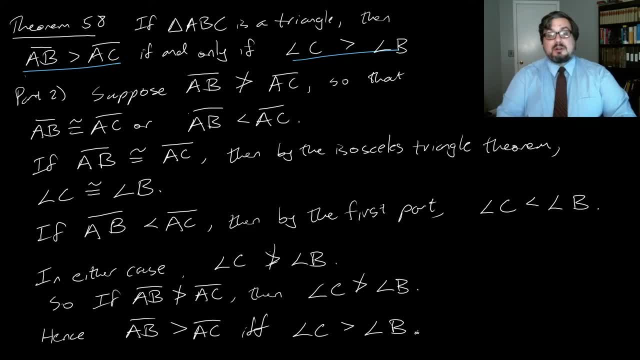 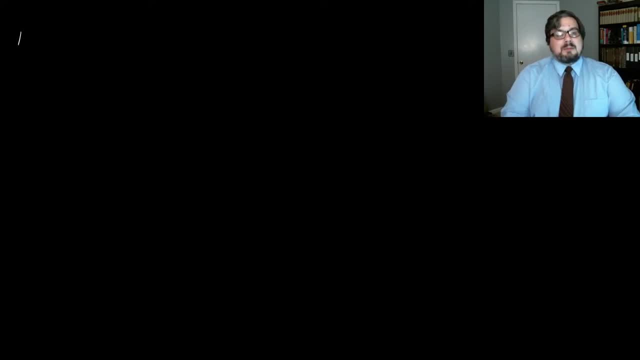 relationship is, then we can get the same statement for either the angles, if we can know the segments, or the segments, if we know the angles. We've got a couple of applications to this. Theorem 59 tells us that the shortest segment connecting a point to a line is contained. 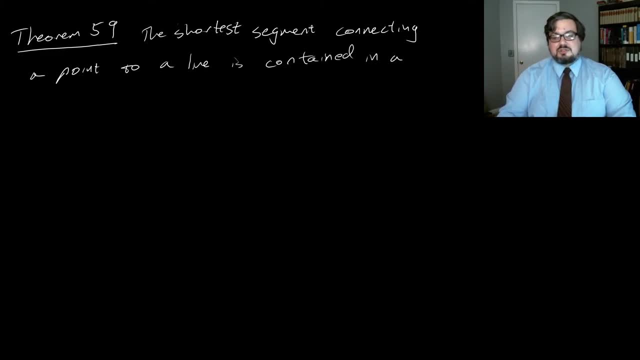 in a line, I should say perpendicular to the first one. So, in other words, if we've got a line and we've got a point, call that point P, call that L, then among all the different ways there are of drawing a segment, we've got a line and we've got a point. So if we've got a line and we've 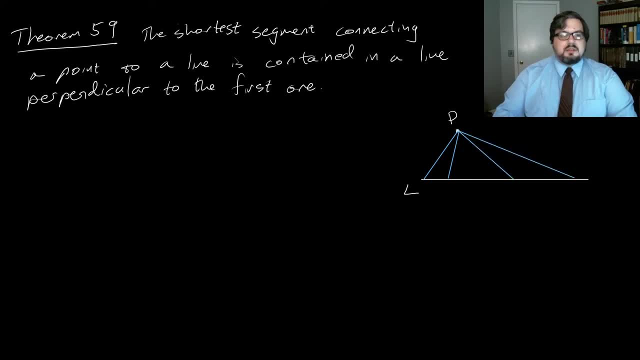 got a segment from P to L, the shortest one is the one perpendicular to it. So in other words, if Q is in L and the line PQ is perpendicular to L and R is any other point of L other than Q, then the segment PR is greater than the segment PQ. 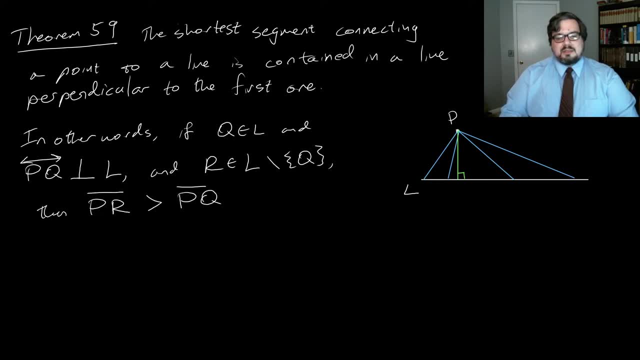 So if we let Q be the point on the line that sits in the line PQ, then the segment PR is greater than the segment PQ. So if we let Q be the point on the line that sits in the line PQ, then the segment PR is greater than the segment PQ. 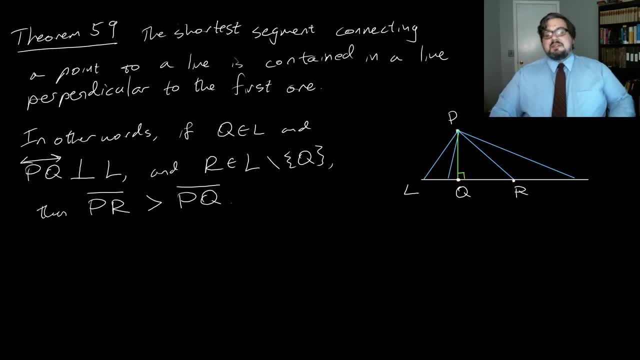 So if we let Q be the point on the line that sits in the line PQ, then the segment PR is greater than the segment PQ. So if we let Q be the point on the line that sits in the line PQ, then the segment PR is greater than the segment PQ. 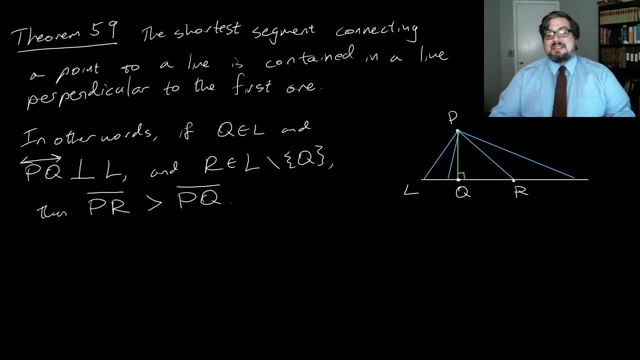 So if we let Q be the point on the line that sits in the line PQ, then the segment PR is greater than the segment PQ. So if we let Q be the point on the line L that sits in the unique line that contains P and is perpendicular to L, 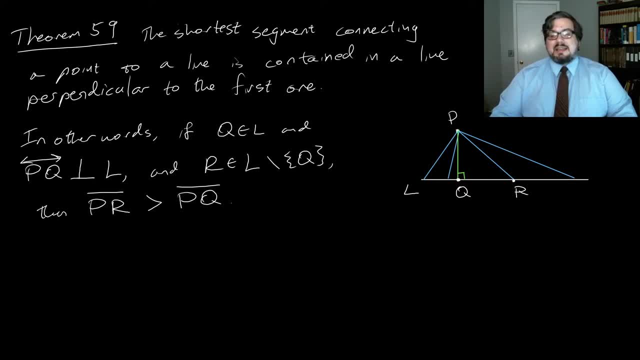 then this segment, PQ, is less than any other segment PR- that we can get on the line. Again, we want to use the stuff that we just had. The actual proof of this is an exercise, However, some hints. you want to construct a picture like this, except, of course, ignore. 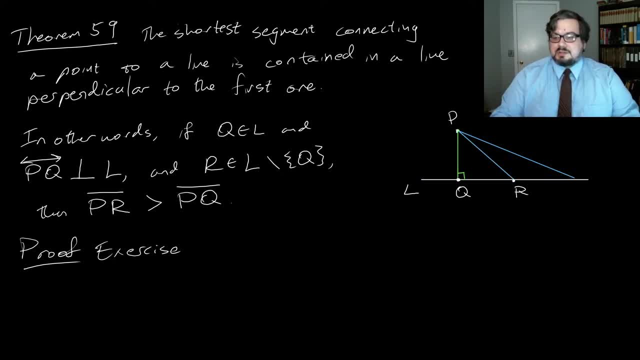 these other extraneous blue lines. you just need to let R be any random, any random point on L other than Q. you want to show that the green line is smaller than the blue line, and so one way of doing that, using theorem 58, is to show: 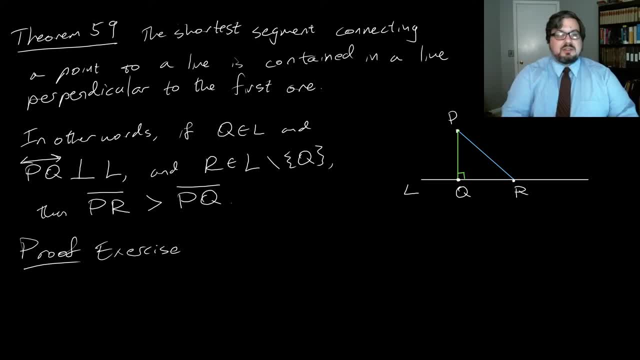 that the angle at Q, the right angle at Q, is less- I'm sorry, greater than this angle at R. now we don't have a direct way of comparing the green angle. I've written to R. however, if you look at this triangle, this red angle is an interior. 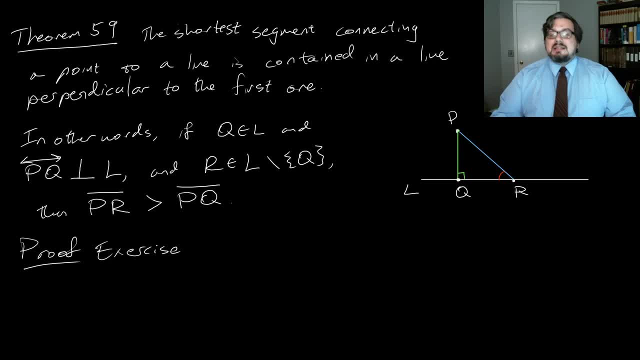 angle, which means that there are exterior angles to this triangle, like that one, which have the red angle as a remote interior angle, and the exterior angle theorem tells us how they're related to one another. so combining the exterior angle theorem with theorem 58- that we just did- will help you to solve this problem. another: 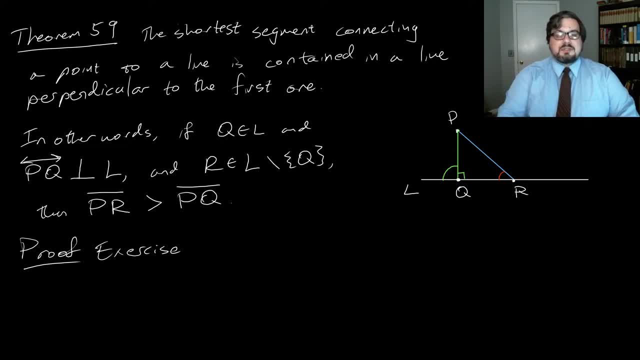 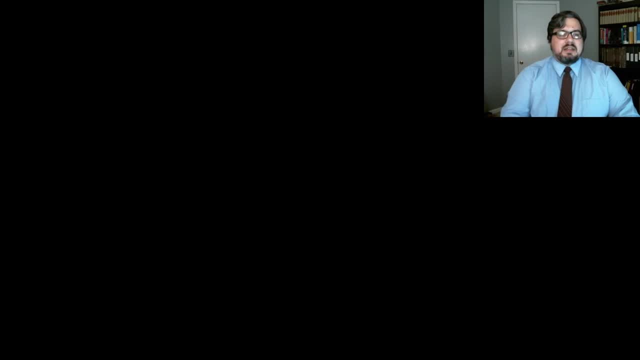 theorem related to the R vector of the triangle R we just did is to show that the these inequalities is often called the triangle inequality. I prefer the triangular inequality because I like to make it slightly more general than it sometimes is. Theorem 60,, which I 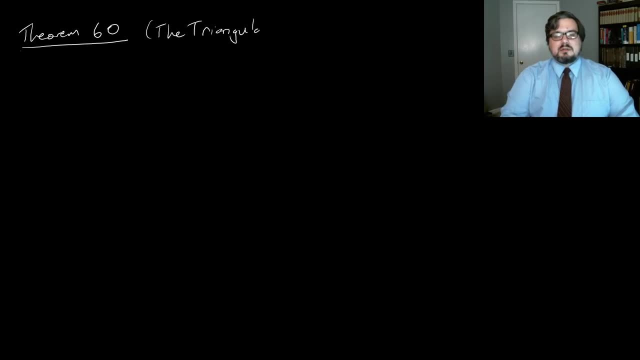 call the triangular inequality says: if A, B and C are any points, then the segment AC is less than or equal to. I'm sorry, not the segment, but the distance from A to C is less than or equal to the distance from A to B. 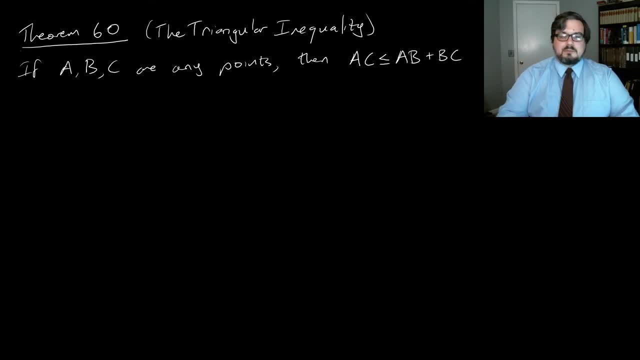 plus the distance from A to C, And equality holds if, and only if, B lies between A and C. So the way to think about this, at least in the non-collinear case, is the following: If I've got three points- A, B and C- 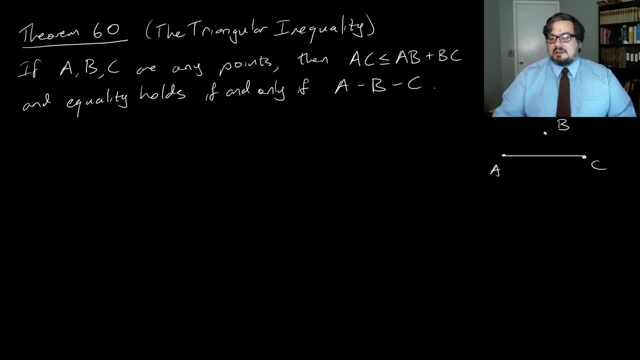 and I look at the distances between all of them, and the figure that I've just drawn shows you why it's called the triangular inequality. the intuition is that the shortest distance from A to C is the line that goes directly from A to C If we take any sort of detour. 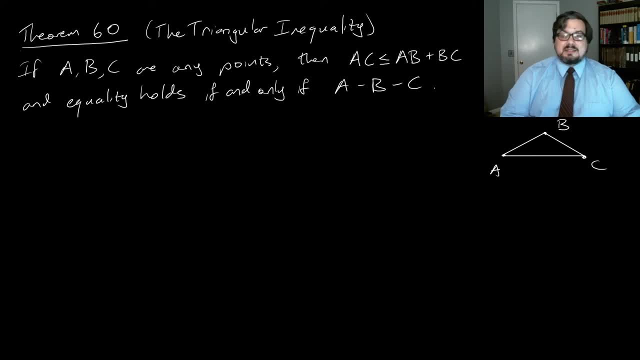 the only thing that can do is lengthen the distance. So if I go straight from A to C, that distance has to always be less than or equal to the distance that I travel going from A to B and then from B to C. 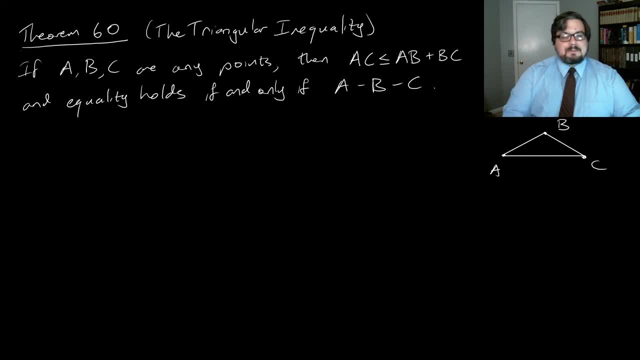 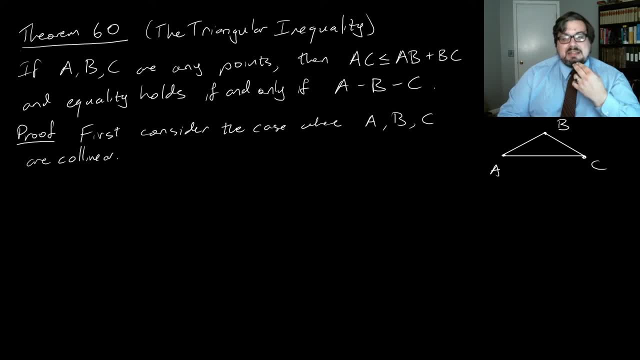 the case that some of A, B and C are equal to one another. If A equals C, the result is trivial, since A C equals 0, and so 0 is definitely less than or equal to A B plus B C, no matter what B is If A does not equal C but- or- let me sorry, do this a different. 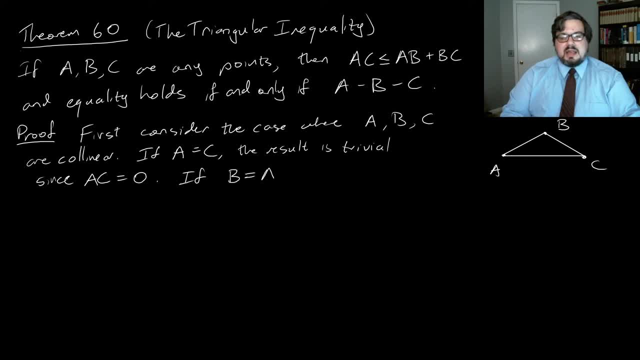 way, If B equals A, or then we have that A, B plus B C is equal to 0 plus now the distance from B to C would be the distance from A to C, which is definitely greater than the distance from A to C because it's equal to it. 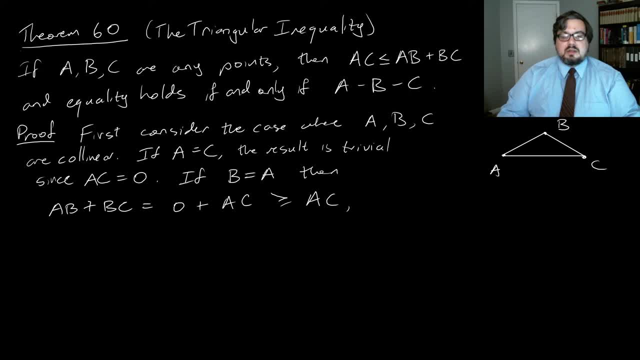 So sorry, I realized a slight technicality in the way that I, the way that I stated this, So let me let me clarify this. So, in the statement, equality holds if, and only if, A, B is between A and C. 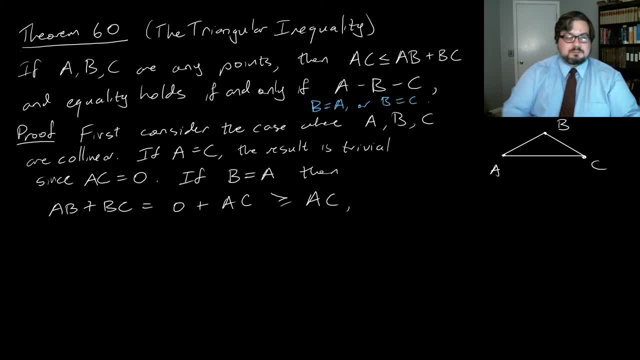 So if B equals A, then we certainly have this situation where A B plus B C is equal to A C- the equality that we were looking at- And similarly, if B equals C, then A B plus B C is equal to A C. So if B equals A, then we certainly have this situation where A B plus B C is equal to A C, And similarly, if B equals C, then A B plus B C is equal to A C. 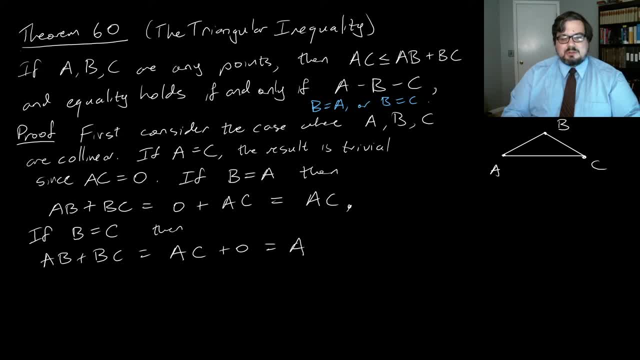 So if B equals A B plus B, C is equal to A C plus 0, which equals A C. So this handles all the cases where any two of the points are equal to one another. So now if A, B and C are distinct but still collinear. 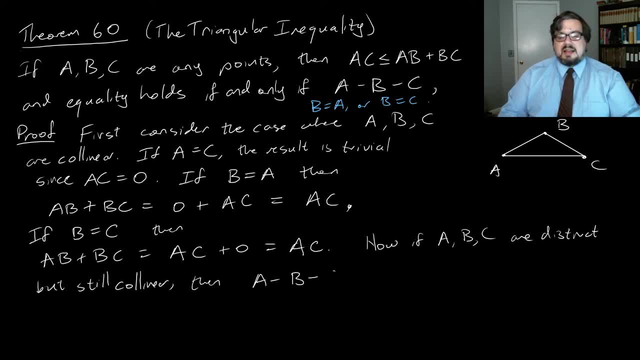 then we have that B lies between A and C if, and only if, A B plus B C equals A C by definition. And so if it is not the case that B lies between A and C, then we may assume without loss of generality: 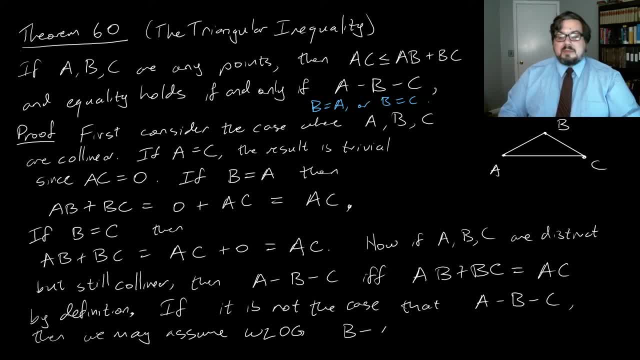 that A lies between B and C, In which case we have that A B plus B C is equal to A, B plus A, B plus A C, Because if A lies between B and C, that means that B? C is equal to B? A plus A C. 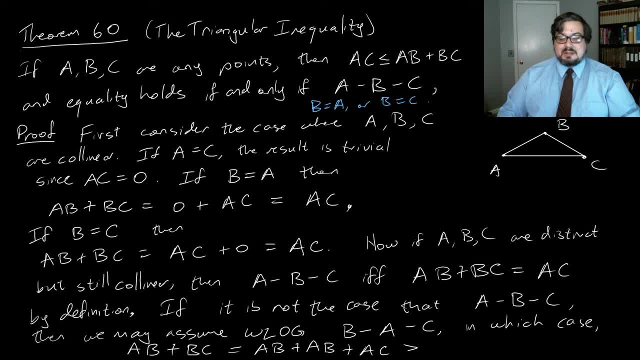 And, in particular, this is definitely greater than A C, Because the distance from A to B is non-zero in this case. So we've shown that in the case where points A, B and C are collinear, first of all, we showed that if any, if any two of them, 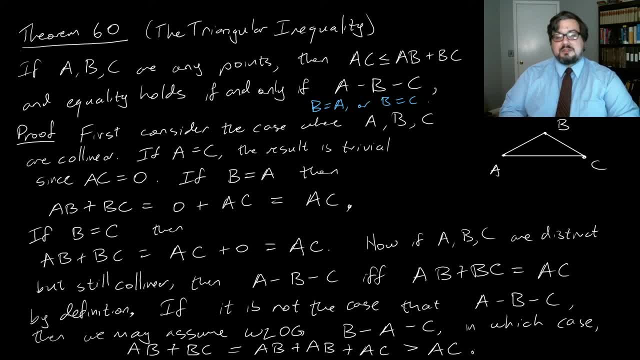 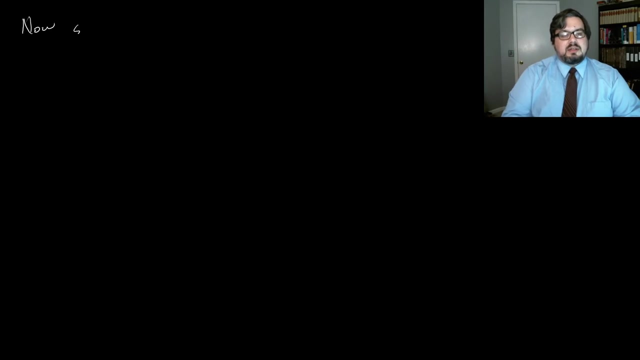 are equal to one another, then we get the inequality that we want, or the equality we want in the case that b equals a, b equals c or b lies between a and c. And so we've handled the collinear case. The more interesting case is the non-collinear one. So now let's suppose 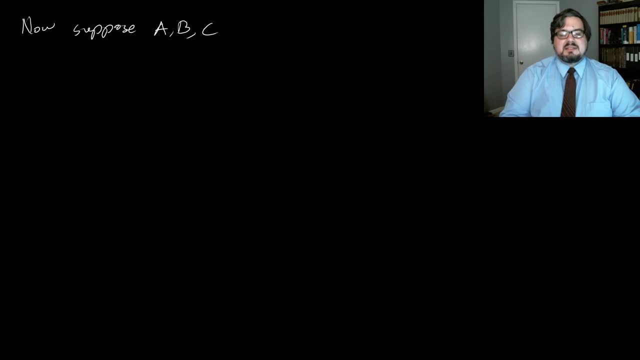 that a, b and c are non-collinear. This is the situation that we had before, So that means that we actually have a triangle here that we can work with a b c. We consider the triangle A b c Now. we want to somehow show that the distance from a to b plus the distance 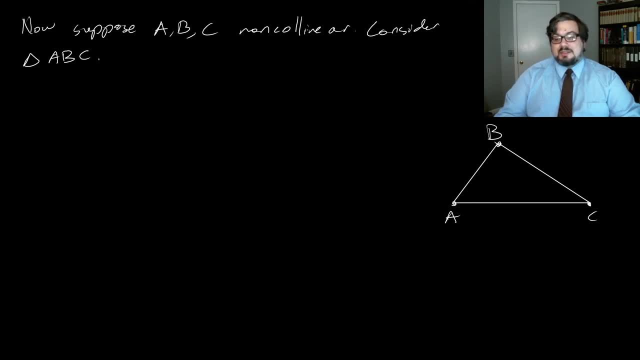 from b to c is greater than the distance from a to c. What we know from our previous theorems is that, if we could, is that we can compare the different sides of a given triangle if we know the distance from a to b to c, And so we want to somehow show that the distance 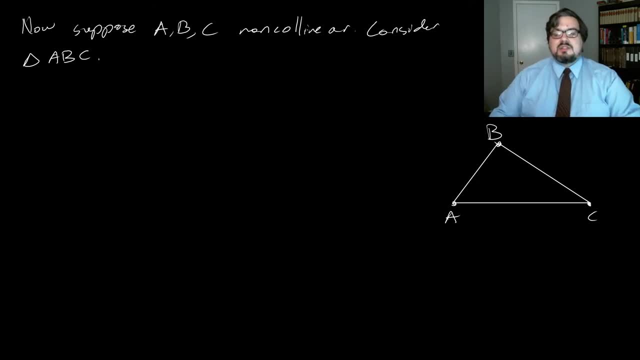 from b to c is greater than the distance from a to b. So now let's do this and check what the depois What we're saying is. I'm not going to write this down, I'm going to just show it in the display, but we want an alternative way to do it. 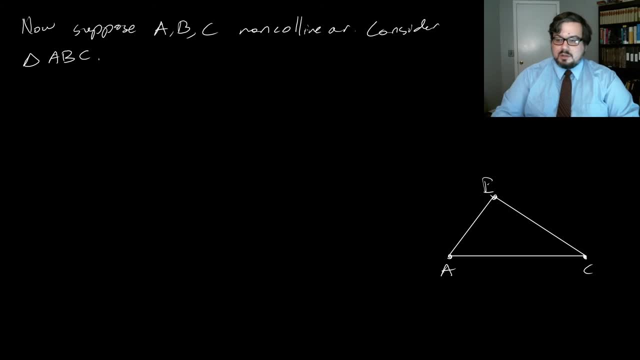 Okay, so there's the 0,, 0 and the 1.. Okay, so now we're in the terms we've measured. I'm going to put down the 0.. So what we took out was this line: endpoint of the terminal. 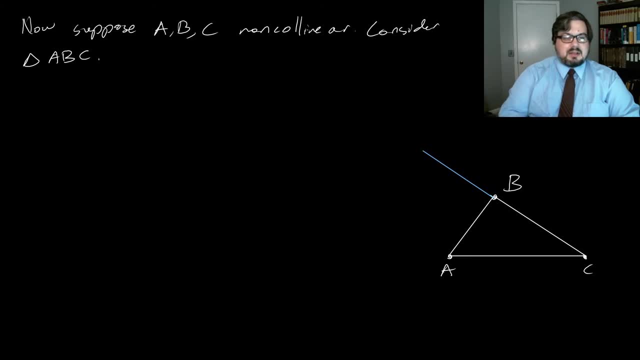 0, 0, 1.. It's going to be 0,0, 1, 0, 0.. segment up like this and we're going to build it in such a way that this distance from D to B is congruent to the distance from A to B. Now what that's? 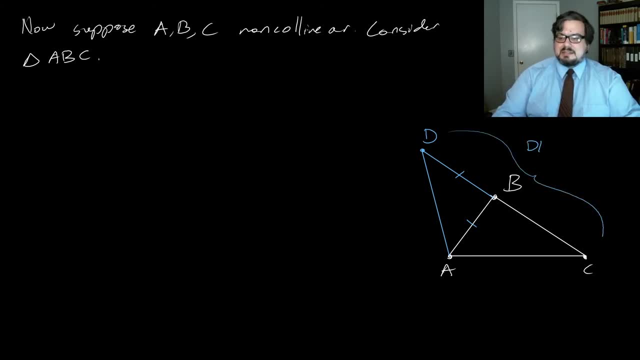 going to do? is it's going to have that the distance DC is equal to AB plus BC, which is what we're looking for? We want to show that that quantity is greater than AC. So what we want to show is that the angle opposite AB plus BC is greater. 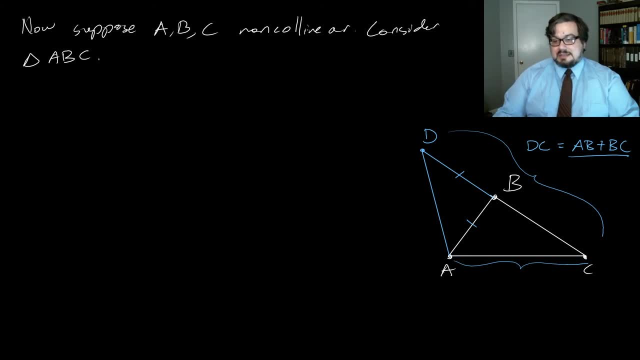 than the angle opposite AC. So let's do this, So let's, let's do this. So let's let B lie between D and C, such that segment DB is congruent to segment AB. So now we've got a couple triangles going on here. So now triangle ABD is isosceles. 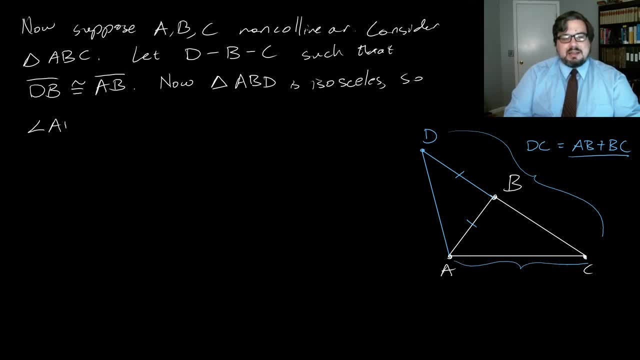 So that means that angle ADB is congruent to angle BAD. We have that these two angles are congruent to one another. Now, since B is in the segment DC, B is in the interior of angle DAC. Therefore, angle DAC is greater than angle ABD. I'm sorry. 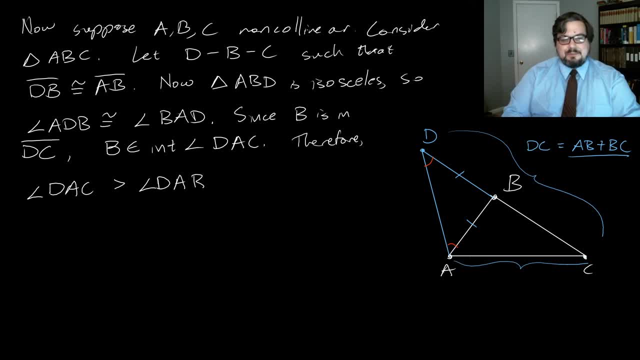 not ABD, Angle DAB, which is congruent to angle ADB. So we have that the green angle, DAC, is greater than the red angles, In particular ADC. By theorem문 58, we have that the segment DC is greater than the segment AC. 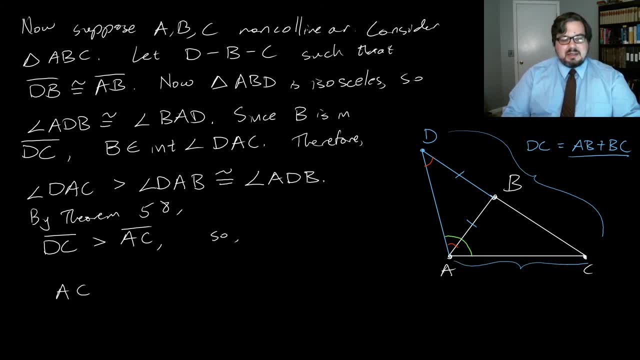 And so this means that the number AC is less than the number DC, and by between this, the number DC is equal to the number DB plus BC, and the distance from D to B is the same as the distance from A to B by construction. 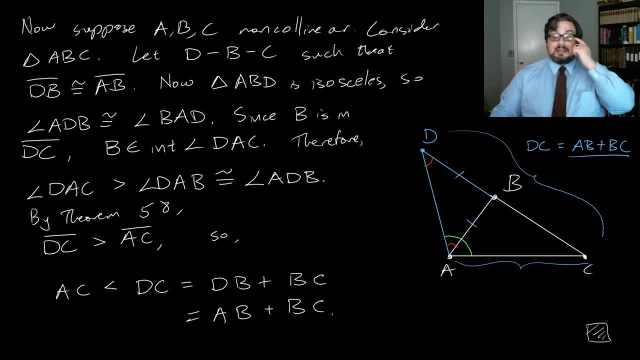 So we proved in the non-collinear case that the distance from A to C is less than the distance from A to B plus B to C. Once again, we did this by copying part of our figure onto another part to make things helpful to us. 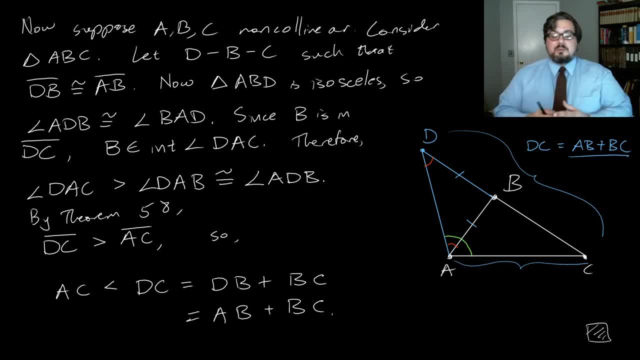 A lot of times We are going to be working with figures and wanting to compare things and a lot of times, if you want to compare sums of distances, it's helpful to arrange all those distances on a single line, to copy them over the way that we copied over the segment AB onto the line BC. 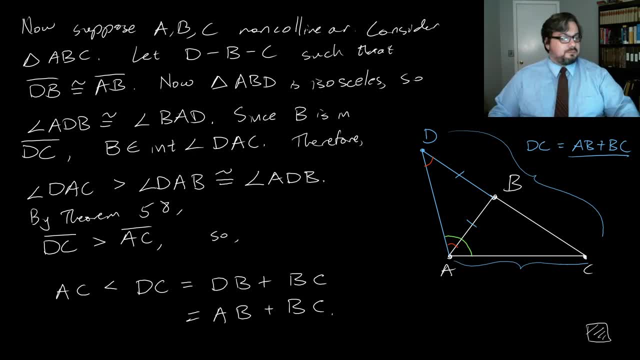 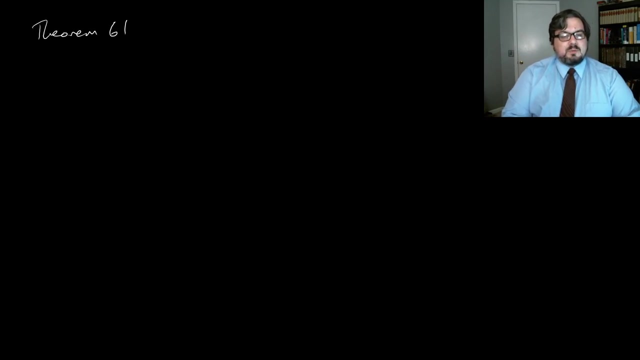 by putting that point D up there. Okay, a couple more theorems we want to look at here. The first one is a generalization of the triangular inequality that we get by an easy application of induction. Theorem 61, I call this the polygonal. 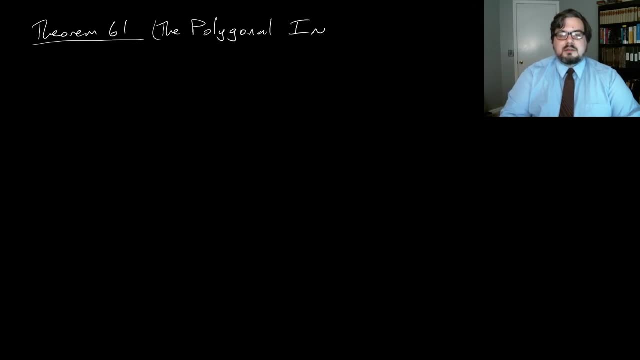 Theorem 61, I call this the polygonal inequality because we're looking at The idea is we're looking at polygons with many sides instead of just three for a triangle. So if A1,, A2, up through AN are points, 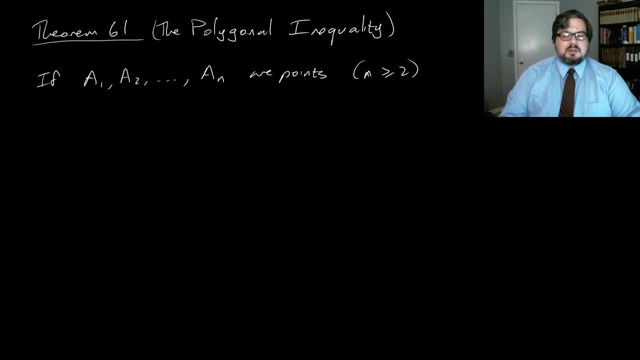 here N has to be at least two. so Then Then The distance from A1 to AN is less than or equal to the distance from A1 to A2 plus the distance from A2 to A3 plus the distance from A3 to A4, etc. etc. 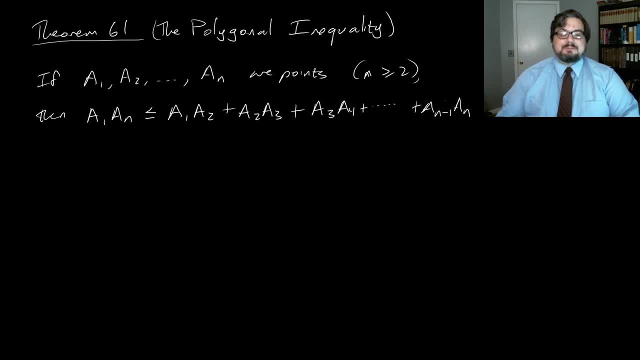 up to the distance from AN minus 1 to AN. The idea behind this is very much the same sort of thing as we did for the triangular inequality. If I've got a bunch of points, A1,, A2,, A3,, blah, blah, blah. 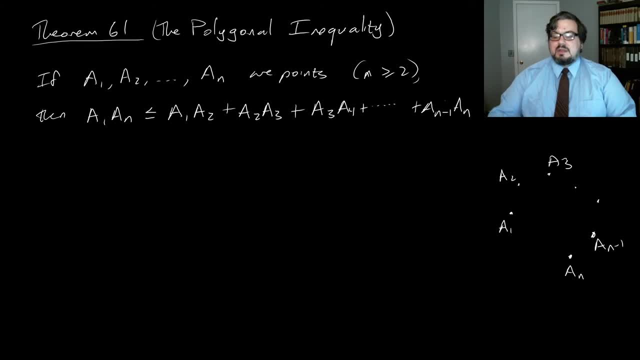 AN, and I'll label AN minus 1 here. Then the path that I take going A1 to A2, A2 to A3, etc, etc, etc, etc, can never be less, can never be shorter than the distance that I get just going from A1 to AN. 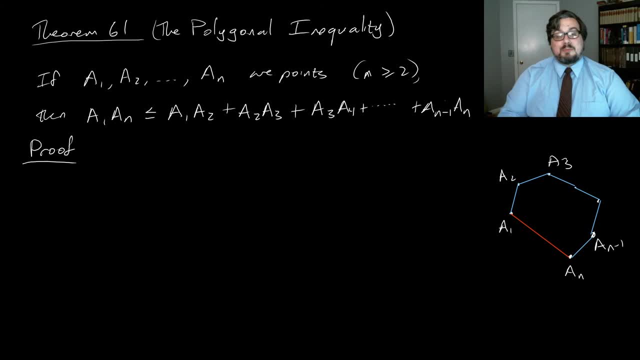 As I say, the proof of this is a fairly easy proof by induction itself. But a stronger proof of this is to get to the título by induction. So our base case. so if n equals 2,, so if n equals 2, then the statement becomes: 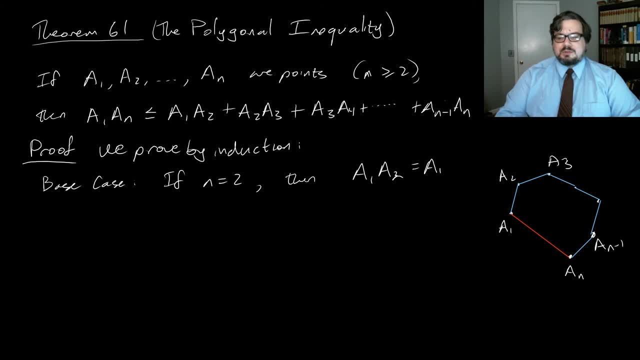 a1, a2 is equal to, is less than or equal to just a1, a2, which is true. So the base case is very trivial. So now suppose we know the result For n, for some n where n is greater than or equal to 2, and we want to prove it for. 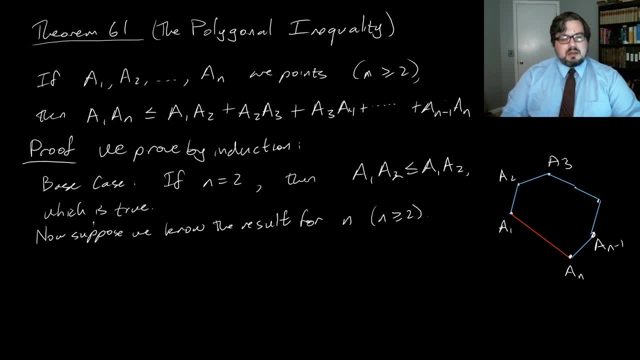 n plus 1.. We have that a1, a2, plus a2, a3, plus, blah, blah, blah, blah, blah, plus. and now we want to show that the sum of these distances up to up through an, an minus, an plus 1, rather, we 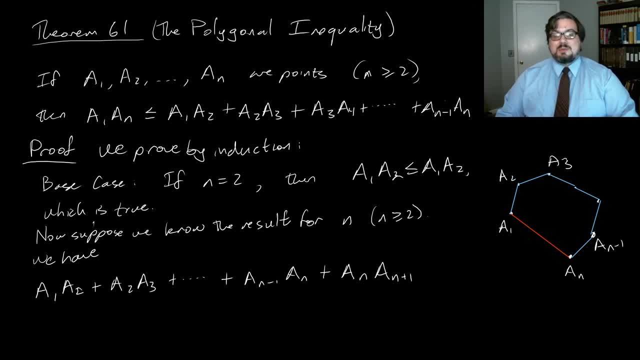 want to show that this is less than or equal to the distance from a1 to an plus 1.. What we know is that we have the result for n of them. So, in particular, we know that all these sums are less than or equal to. 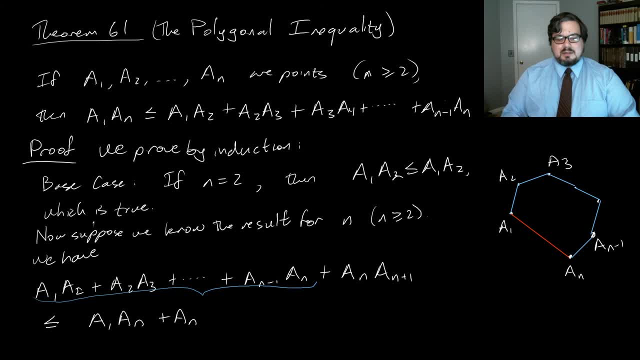 the distance from a1 to an by the inductive hypothesis, and then this is less than or equal to a1, an plus one by the triangular inequality. So the polygonal inequality is not unintuitive and it continues to basically say the same thing that the triangular inequality. 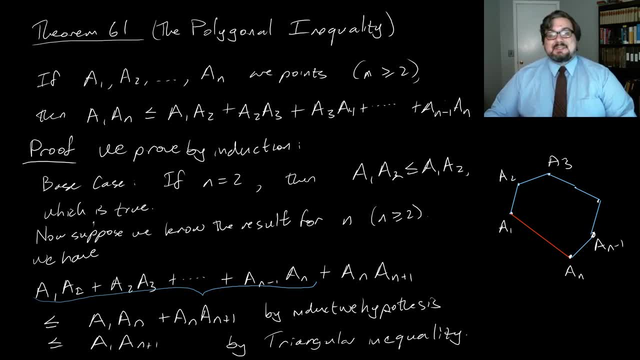 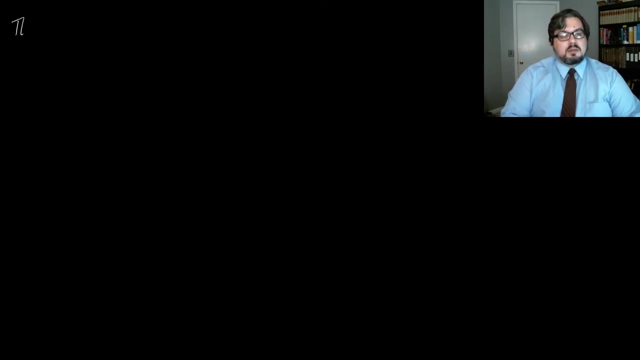 did, which is that the shortest distance between any two points is basically the segment that directly connects them. all right, so now let's look at a theorem that will take a little bit more work but winds up being quite important to us. so theorem 62 is called the hinge theorem. 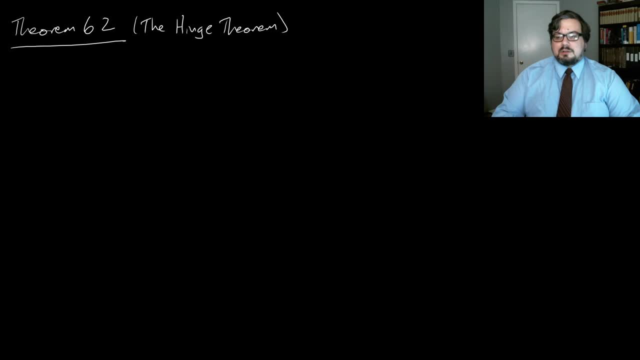 and the basic idea is that we're looking at a couple of triangles. we're assuming that we've got triangles that look something like this: uh, let's actually put in the the sides and we'll label a, b, c, d, e, f and the hinge theorem is going to be: 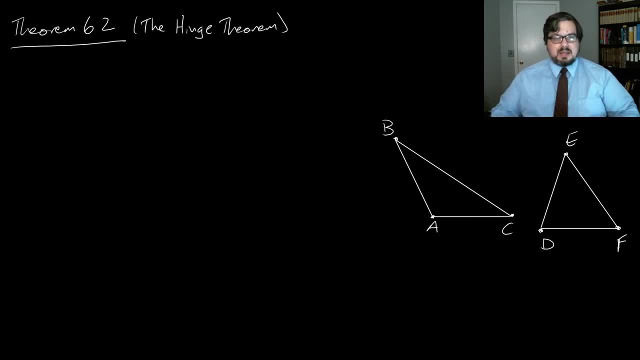 sort of an inequality version of side angle side. we're going to assume that we know that the segment AB and the segment DE are congruent, that the segment AC and the segment DF are congruent, but we're going to assume that the angle at A is greater than the angle at 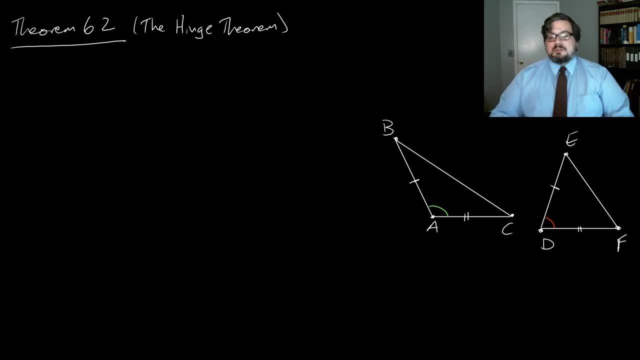 D, Our conclusion is going to be that the distance from B to C is greater than the distance from E to F. The idea behind this proof comes from, or is implied by, the name. If I've got a hinge, then the idea is that as I open the hinge further and further up the distance. 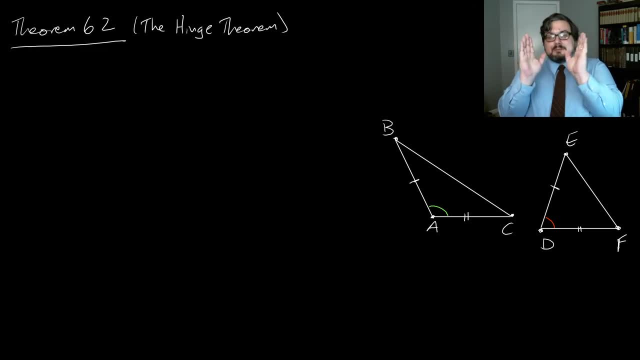 between the two endpoints of the flanges will get bigger as we open it up, And that is what the hinge theorem is. So the statement is the following: Given triangle ABC and triangle DEF, if the segment AB is congruent to the segment DE, the segment AC is congruent to the segment DF and the 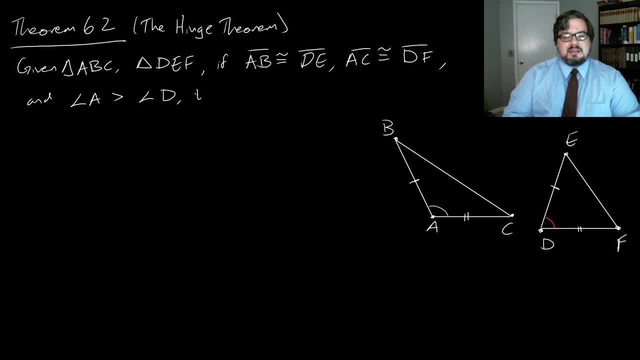 angle at A is greater than the angle at D, then the angle at AB is greater than the angle at D. So, as I say, it's sort of an inequality version of side-angle-side, because we're assuming that we've got a couple pairs of sides that are congruent, but then the angle 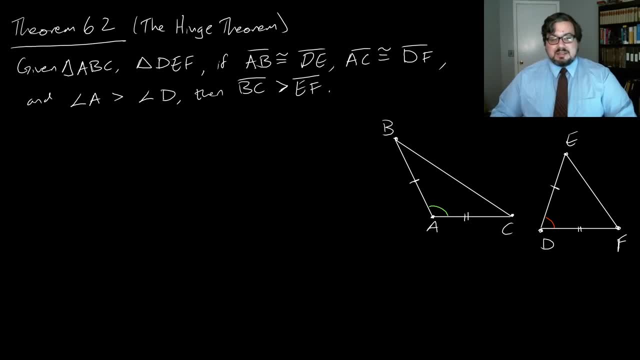 in between is not congruent but has an inequality that we know the direction of. Okay, as normal, we are going to construct a copy of the triangle on the right over here, triangle DEF, over onto the triangle ABC, to work with and start comparing things to. 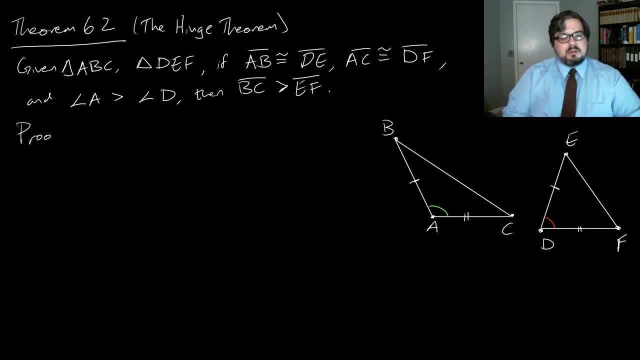 So, since the angle A is greater than angle D, there exists a ray AG. Let's see AG, Yes, A ray AG with, With G in the interior of angle A, such that, Yes, Such that the angle GAC is congruent to the angle FD. 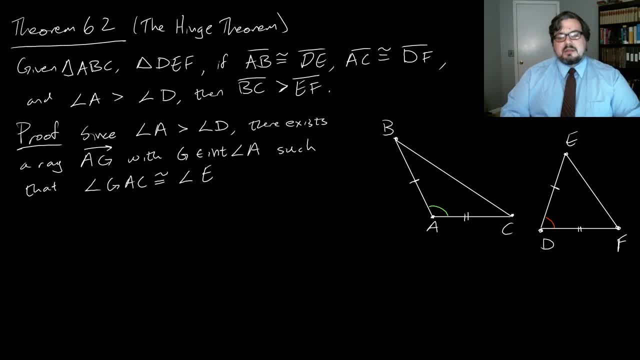 Let me keep the point straight, EDF. So this is saying that we can create a copy of, Or we can copy part of, the ray Or the triangle DEF over here, and we know this because of the hypothesis that the green 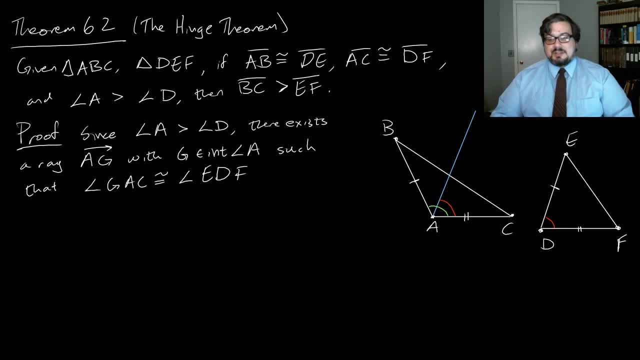 angle A is greater than the red angle D. By definition that means we can construct a ray like this. Now by the crossbar theorem We have that the ray AG intersects the segment BC Without loss of generality. We may assume that G is actually in the segment BC. 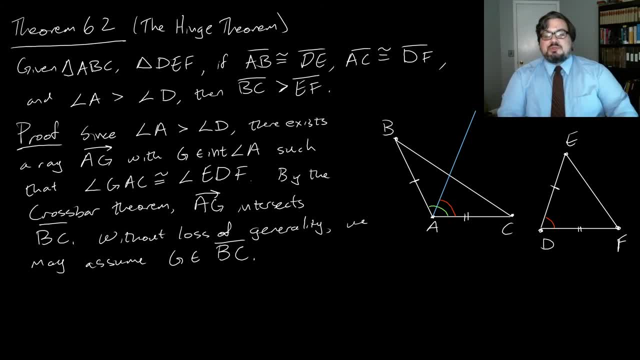 So far, we haven't done anything with G. We've only used G to indicate the blue ray, And so that means that we can, Instead of choosing G, we can choose whatever point. Whatever point, this is where the ray actually intersects the segment BG. 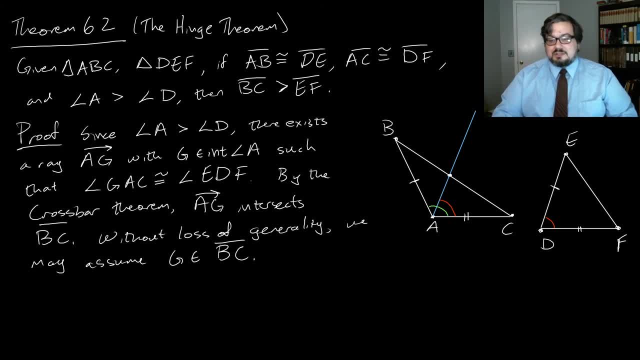 And once we do that then we can basically just relabel it G, because the original point that we had doesn't really carry any meaning. So we can explicitly choose. Let's just make G be the point where this ray AG intersects the segment BC. 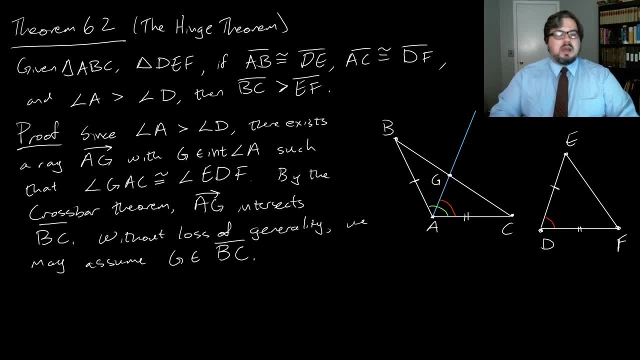 Oh, I apologize. I want to make sure to not deviate from the notes in the book too much, And so let me replace all my G's with H's, I beg your pardon. So let's just Let's make that point. H. 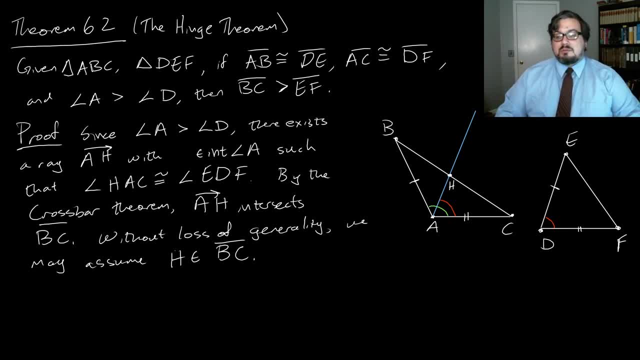 Because what I want to do is I want to use G to represent the point on the ray Where the segment DE is congruent to the segment AG. So let G be in the ray AH, such that the segment AG is congruent to the segment DE. 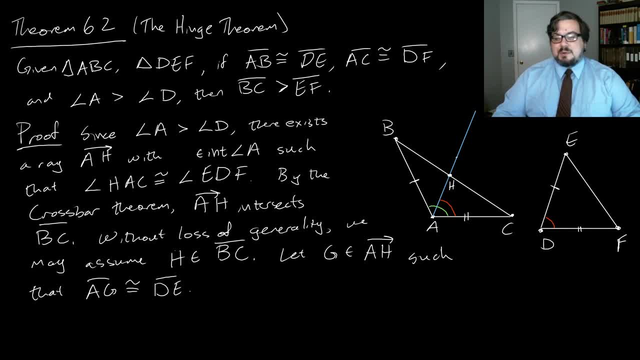 So now we put a G on the blue ray. Now here's where we need to be a little bit careful, Because there are basically three different places that G could be. So let me not even put it in white, Let me. 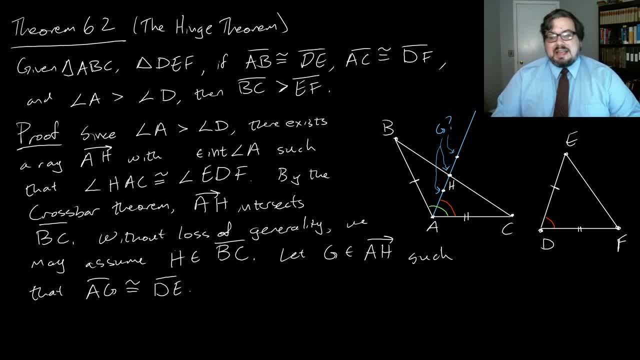 G could be in basically one of these three cases: We could have that G lies between A and H. We could have that G is actually equal to H. Or we could have that G lies on the other side, That H is between A and G. 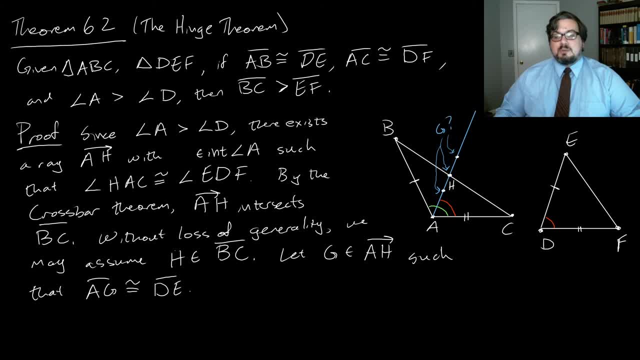 As it turns out, our argument works perfectly well for both of the G's that aren't equal to H. If We'll have one argument that works if G is either between A and H or H is between A and G, And then we're going to need to have an argument for what happens if G is actually equal to H. 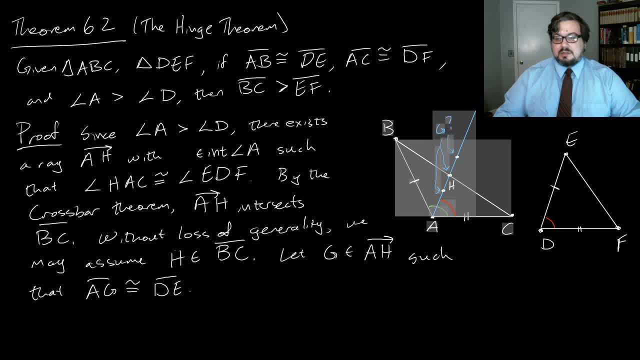 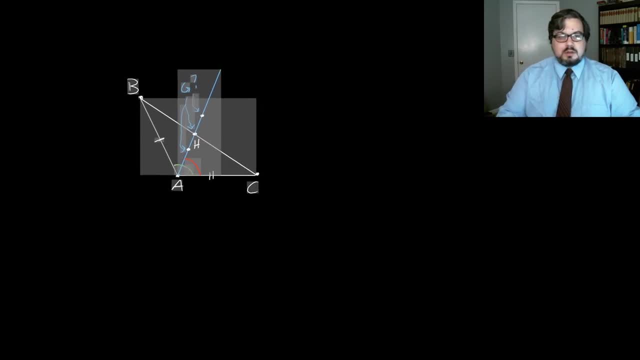 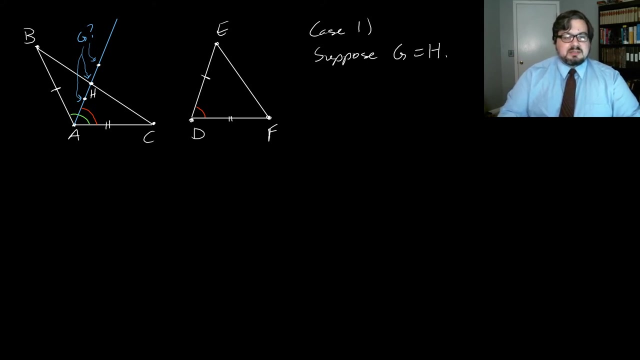 So let's get a new page And look at those arguments. Oh, and we're also going to need the triangle DEF. So let's continue. So case one: Let's suppose that G actually is equal to H. So let's suppose G is equal to H. 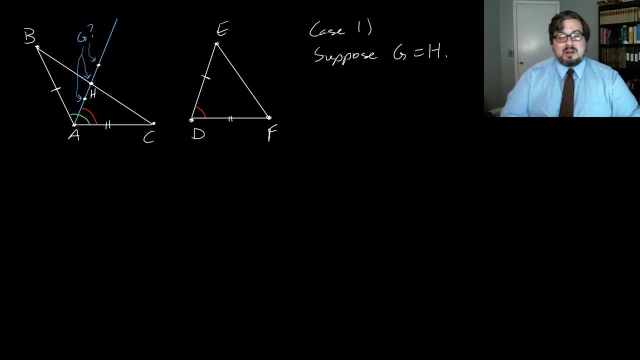 And so that means that the segment AH is congruent to the segment DE. So segment AH is congruent to the segment DE. Thus, this means that triangle AHC- AHC- is congruent to the triangle DEF by side-angle-side. 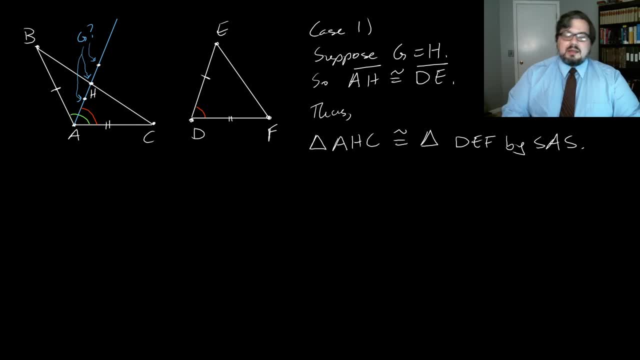 And then, since, Since H lies between B and C, that means that the segment BC is greater than the segment HC, Which is congruent, by this congruence that we have up above, with the segment EF, Which is what we were trying to prove. 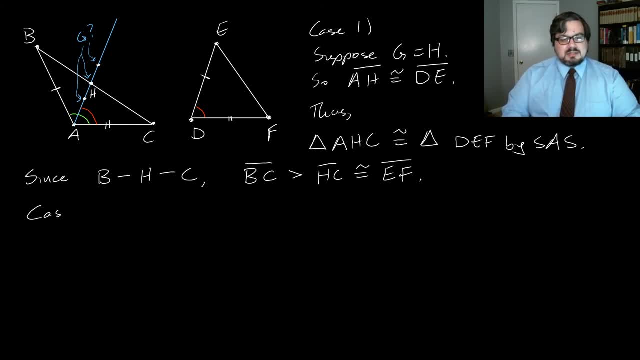 So case one is handled there. So let's consider case two. So for this let me get rid of these, And I'm going to sketch out the proof, assuming that G is sort of on the outer Side here. 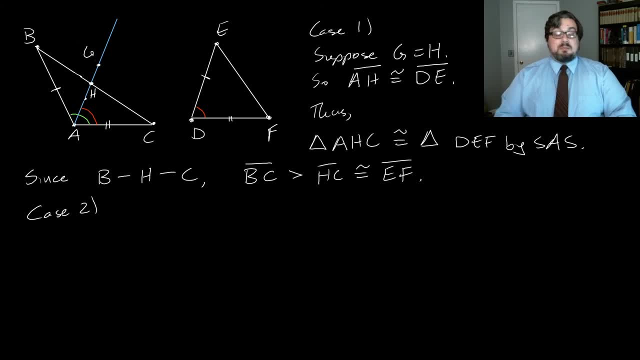 But it's going to turn out that the proof that we write down applies perfectly well, even if G is between A and H. So let's just suppose that G is not equal to H. So here we're going to need to continue to. 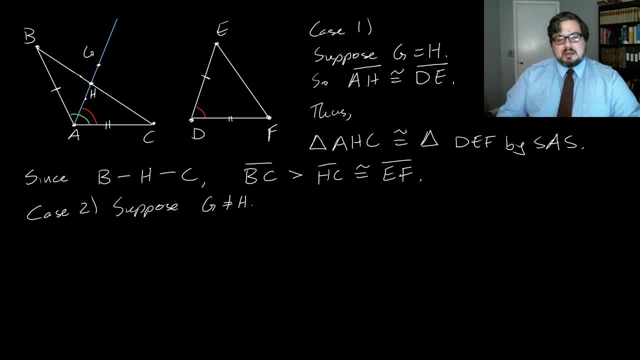 To work some more here. So again, by the crossbar theorem, There is a ray AJ. I'm sorry, not there is a ray. By the crossbar theorem, the bisector AJ of angle BAH intersects the segment BH, say at J. 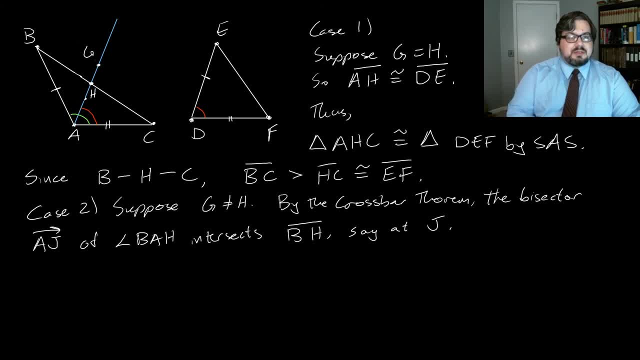 Without loss of generality, we can assume that this bisector here Intersects the, The Segment BH at J. Now we've set this up so that J, The ray AJ, is the bisector of the angle BAH. So now, 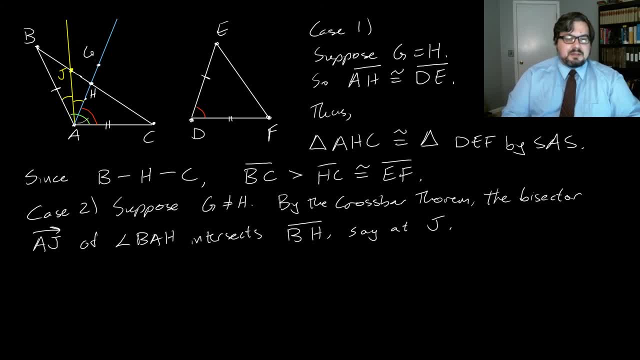 Look at the following. We have that the segment AJ has a single tick. It's congruent to the segment AB, Which means that if we draw in the segment from J to G, Then we've got the two triangles BAJ and GAJ. 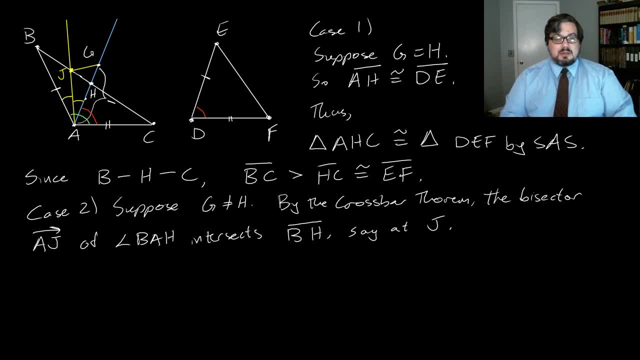 And those are going to be congruent By side, angle side. The segments BA and GA are congruent to each other by construction And the segment AJ is congruent to itself And the angles BAJ and GAJ are congruent because 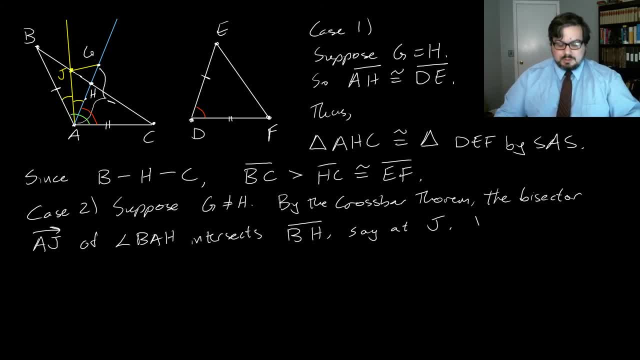 AJ is the bisector of that angle. So, all told, we have that by side angle side, We have that triangle BAJ is congruent to triangle GAJ, And so We have that the segment JB is congruent to the segment JG. 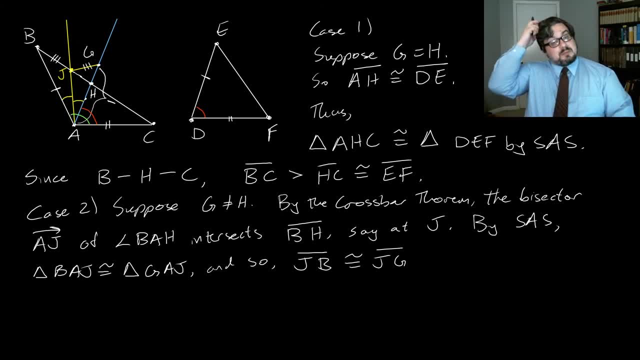 So We have that those two segments are congruent because They are corresponding sides in congruent triangles. So now By the triangular inequality We have that The distance from C to G, We're bringing in some more, Some. 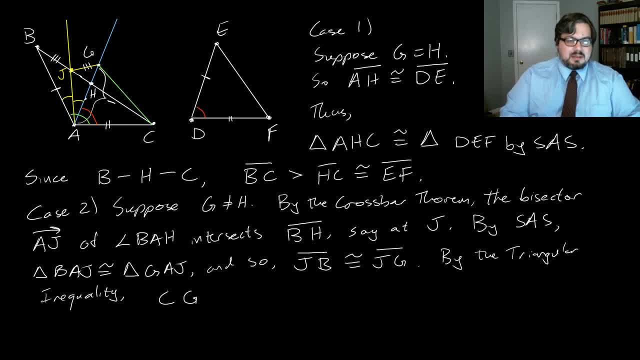 Some more stuff now. From C to G Is Less than the distance from C to J Plus the distance from J to G. We have that the distance from J to G Is equal to the distance from J to B, Now, because J lies in the segment BC. 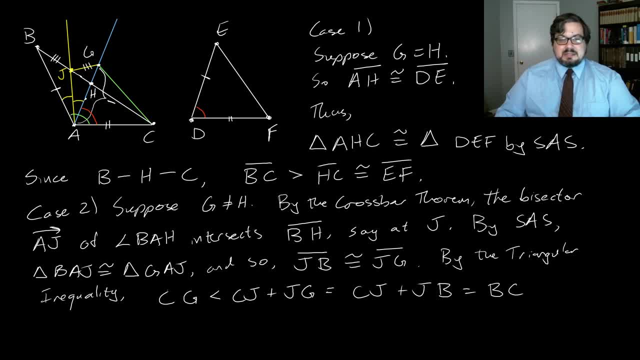 J is between B and C, So this is BC. Now We have that. the triangle AGC Is congruent to the triangle DEF By side angle side. This is actually the same as we did back in case one. 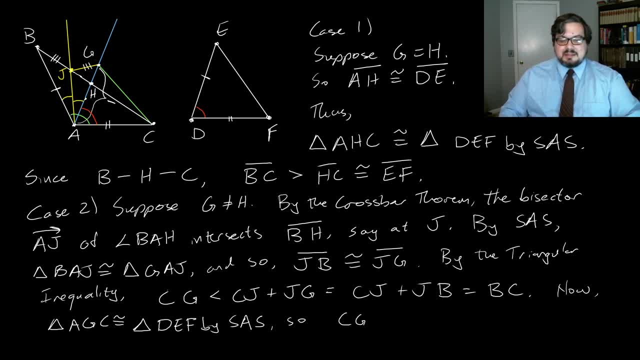 So that means that The segment CG Is congruent to the segment EF. Therefore, Segment EF Is congruent to the segment CG, Which we just showed is less than Segment BC. And that finishes it off. This was. 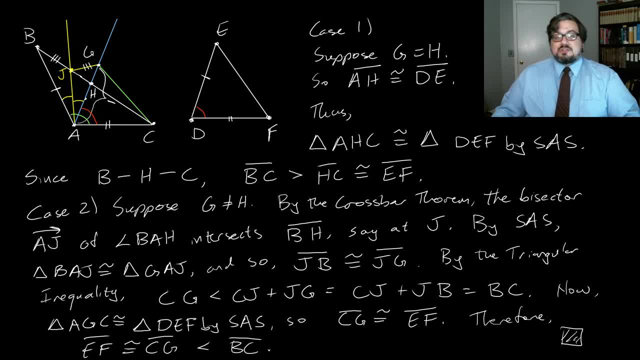 This was so far Our most complex construction And it's really non-intuitive. It's Not the sort of thing that One would easily come up with. Some of the constructions we do are Fairly straightforward, Fairly natural. 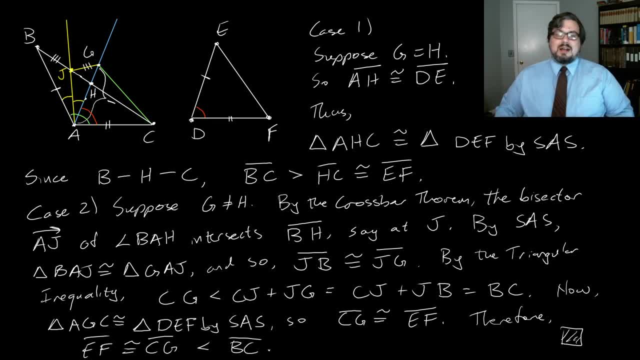 Once you've- Once you've worked with the geometry for a while, This one is Is pretty clever. This is not one that You would come up easily with, Even with a lot, of, A lot of time Spent on it. 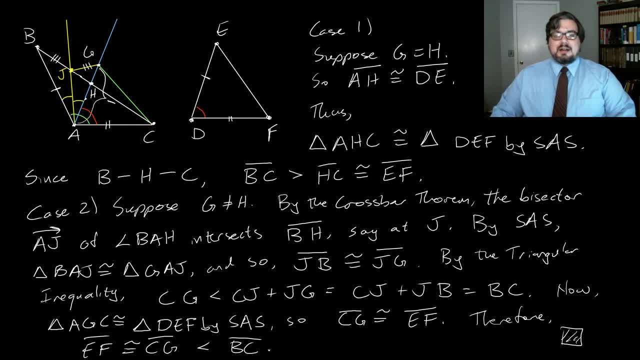 So It's good that we have had Other Other people to Go before and find the Efficient proofs of these Very useful theorems. So Just two more statements here, One of them as an exercise That I want to give a hint on. 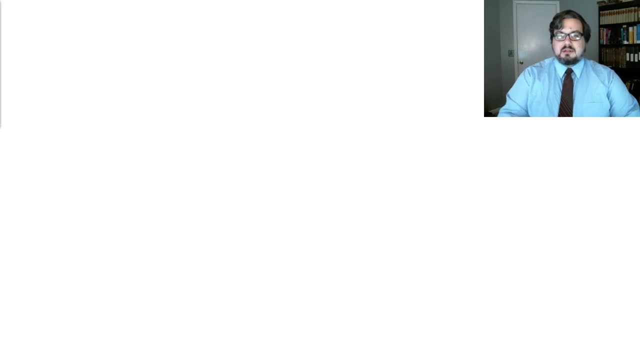 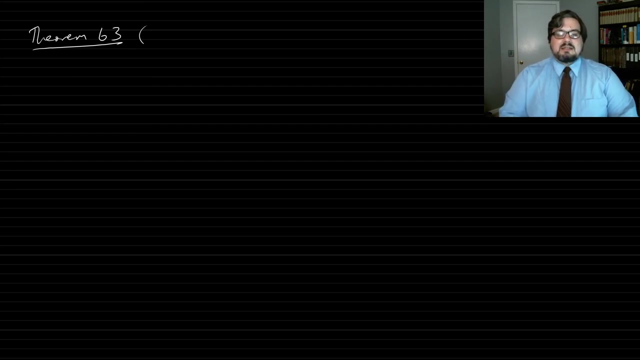 So, Oh, sorry about that. So theorem 63. Is our last. Sorry about that, I'm not sure what's going on here. Theorem 63 is our last Congruent statement for triangles for a while. This is side angle angle. 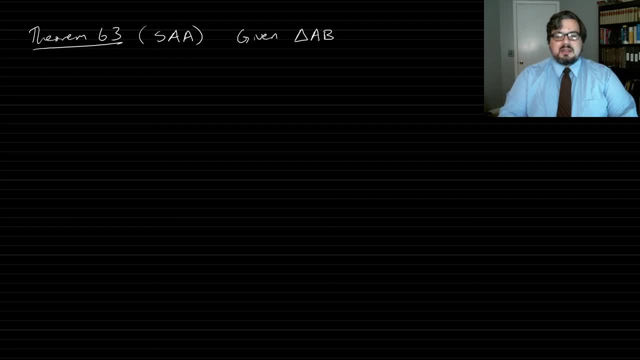 And It says that, given triangles ABC And DEF, If Segment AB Is congruent to segment DE, Angle A Is congruent to angle D And angle C Is congruent to angle F, Then Triangle ABC Is congruent to triangle. 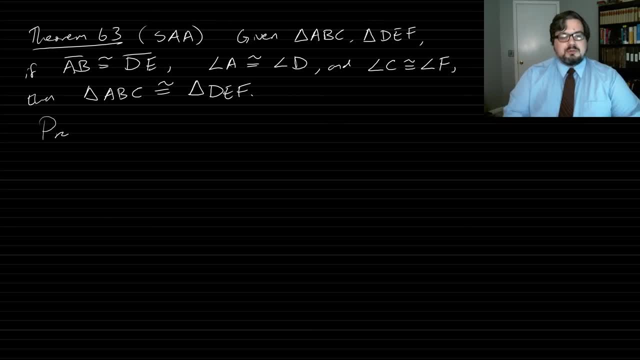 DEF. The proof Is an exercise, But here's, Here's something to get you started on it. So We've got a couple of triangles And Let's see, We've got A, B, C, A. 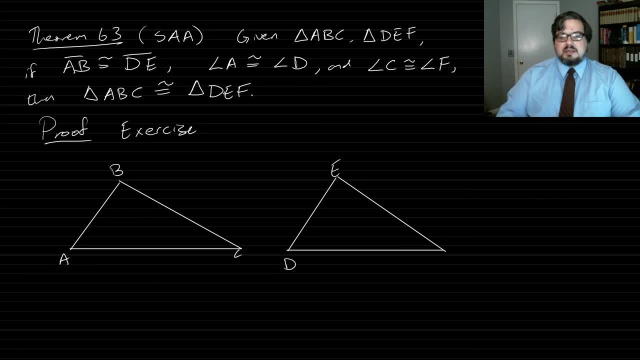 Not A, D, E, F, And We're told that AB Is congruent to DE. So we have This congruence here. We have that angle A Is congruent to angle D And We have that angle C. 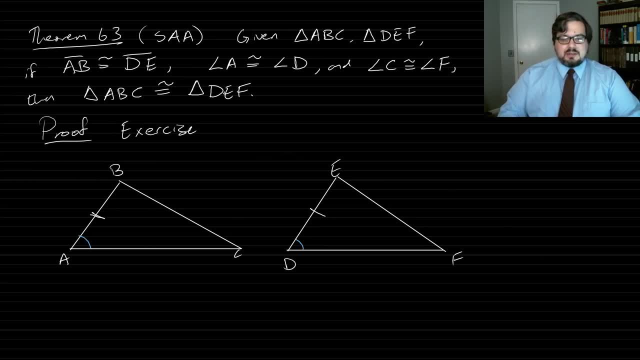 Is congruent to Angle F, And We have that angle C Is congruent to Angle D, Is congruent to To angle F, And We want to show that angle ABC Is congruent to Triangle ABC. 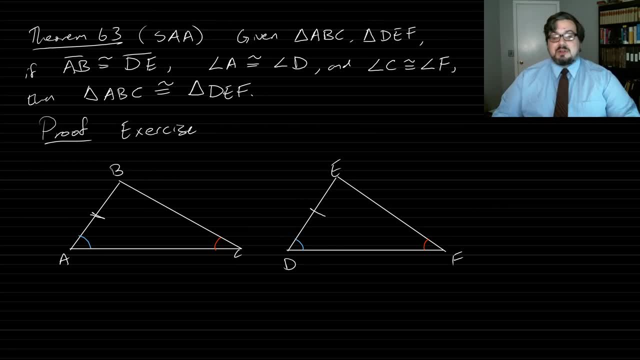 Is congruent to triangle DEF. Now, As normal for these types of problems, You Want to Use Side angle side Or Side side side Or one of the other Results. at some point In this case You probably want to use. 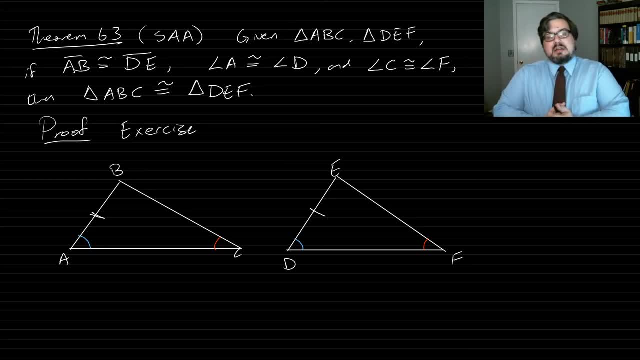 Side angle side, Because you already know something about angles. So We're going to use Side angle side Or Side side side Or One of the other Results at some point. So The way to get started on this. 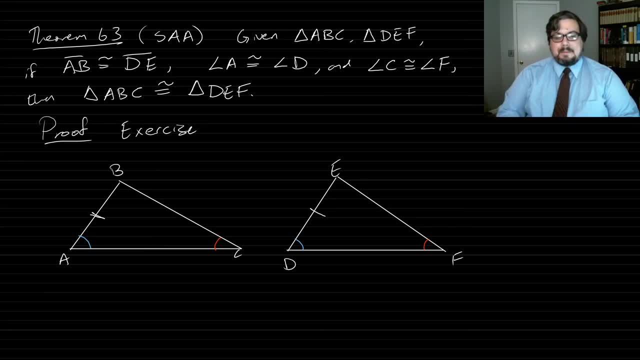 Is to Basically Copy over The triangle ABC Onto the triangle DEF Or vice versa. So What you might do Is Something like: Let C prime Be in the ray DF, Such that The segment AC 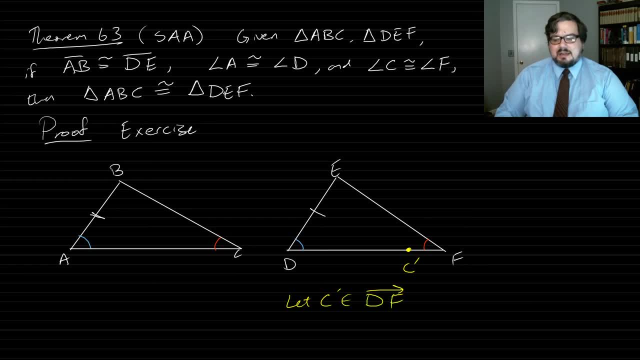 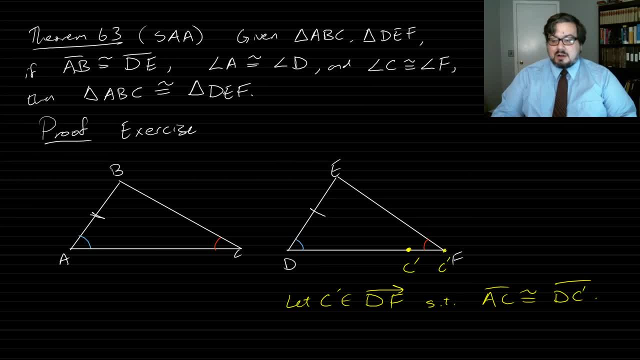 In the You've done before with your other ones. Now Be careful here. There Are Three possibilities. When you do this, You could have the C prime Lies between D and F. We could have the C prime equals F. 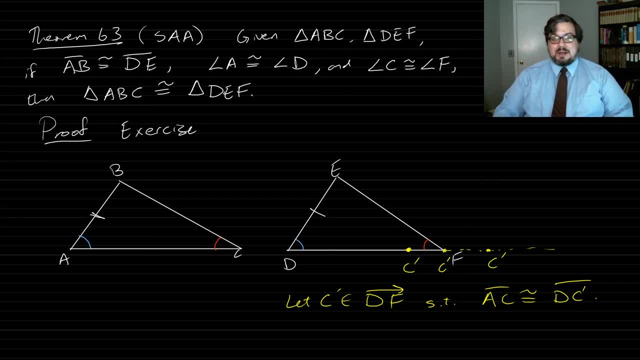 Or the C prime Is On the other side, That F lies between D and C prime And Technically You need to handle These cases. Now what you really want to show Is that C prime is equal to f, because once you've determined that c prime, that a c is congruent to d c prime, 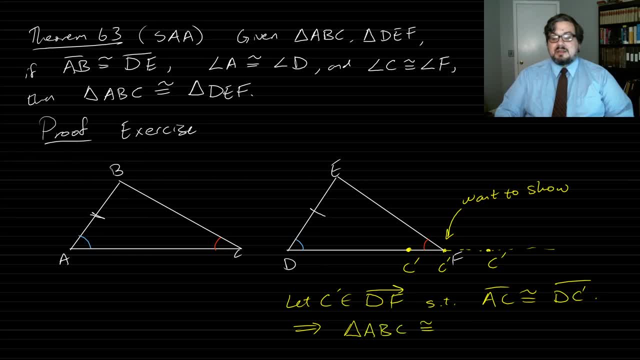 you'll be able to conclude that triangle a, b, c is congruent to triangle d, e, c prime. So you want to show that c prime is actually equal to f. So one way you can do that is to show that c prime can't be in either of the other two possible locations. 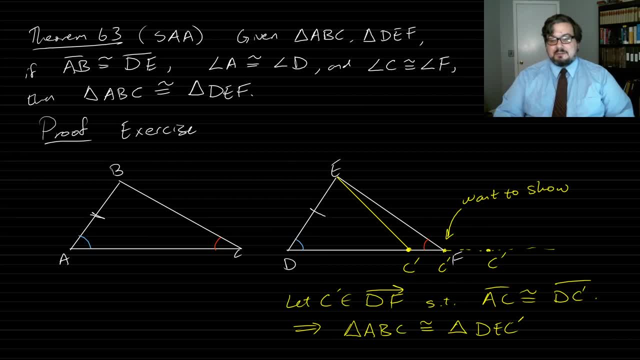 So show that if c prime is there, there's a problem. and show that c prime- if c prime is there, there's a problem. And the trick is to look at is to sketch in d e c prime and then see what happens to this angle when you copy it over to the angle d e c prime. 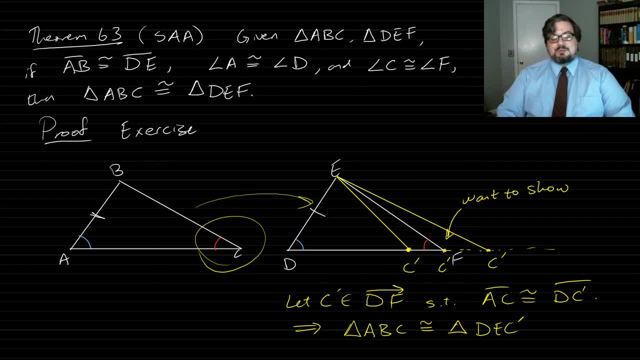 You'll be able to do that. You'll be able to see that this right angle is going to be congruent to some other red angle that we haven't noted yet on the right, which will give you a contradiction if c prime is not equal to f. So that's how to get started on side angle angle. 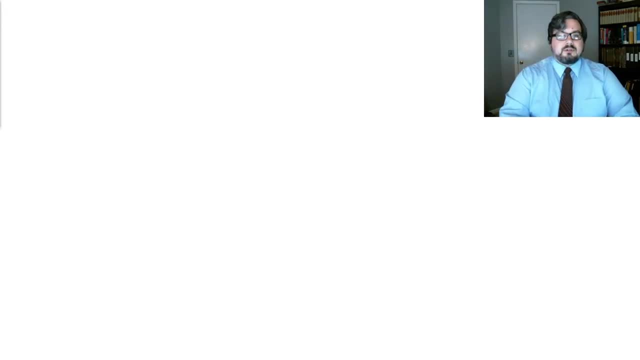 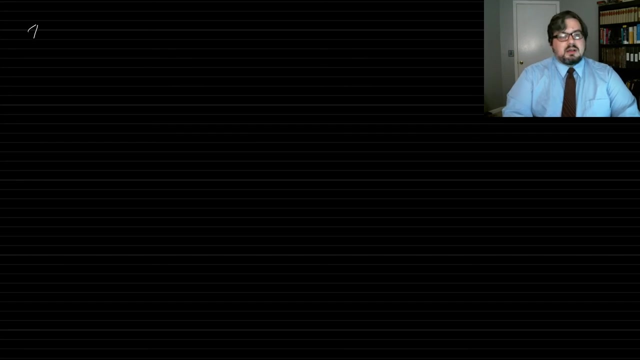 All right, last result for right now. I'm sorry, I don't know what's causing these problems. Theorem 64 is called the hypotenuse leg theorem. Now, before we get into the hypotenuse leg theorem, we're going to talk about the hypotenuse leg theorem. 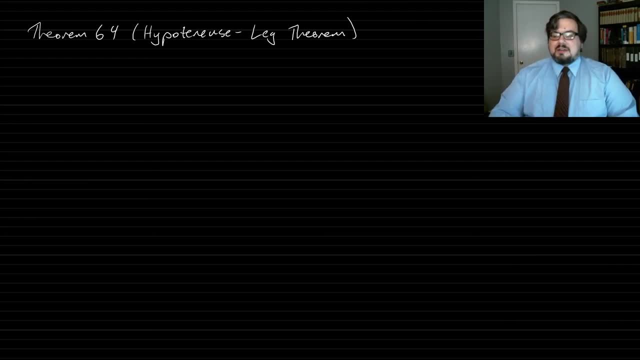 Now, before we get into the hypotenuse leg theorem, we're going to talk about the hypotenuse leg theorem Now before. before stating it, I want to think about the various congruence axioms and theorems that we have. 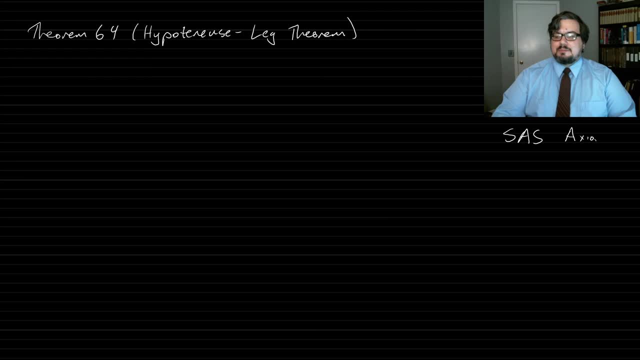 We had side angle side and that was an axiom. And then we proved. then we proved side side side. So that was, that was a theorem. We proved angle, side angle. That was a theorem. We are about to prove side angle angle. 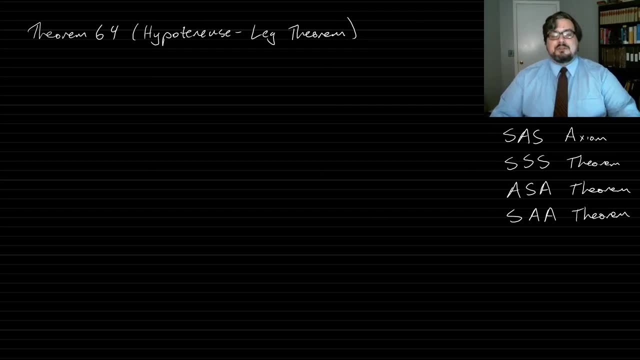 That's a theorem, or rather you are about to in the exercises And there are two more possible theorems that you could have. You could have, you could ask about what if you have side side angle? What if you know that two pairs of corresponding sides are congruent? 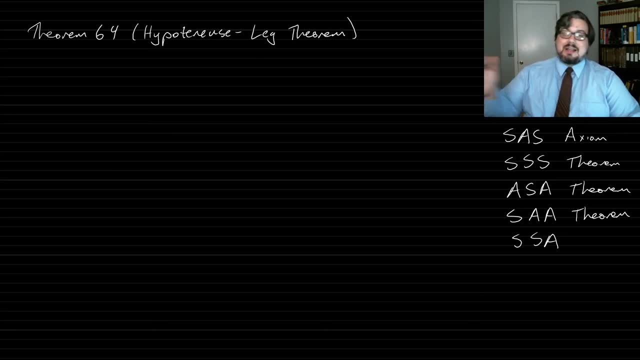 And an angle of side side is the same. an angle is congruent, but that angle isn't between the two sides. And you could also ask about angle, angle, angle. And neither one of these results are actually theorems. If all you 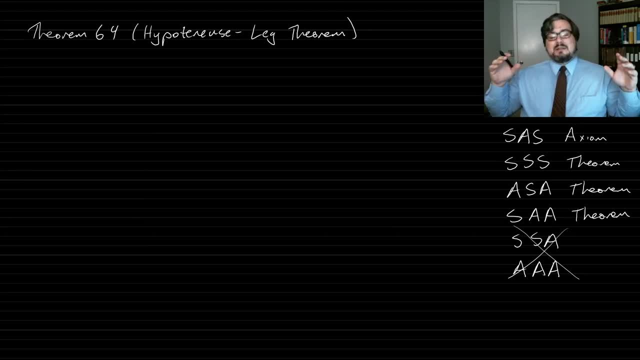 know is that two pairs of sides are congruent and then an angle pair is congruent. if that angle doesn't lie between the two sides, you can't actually conclude that the two triangles are congruent most of the time. Theorem 64 is an exception to this. It's one place where knowing 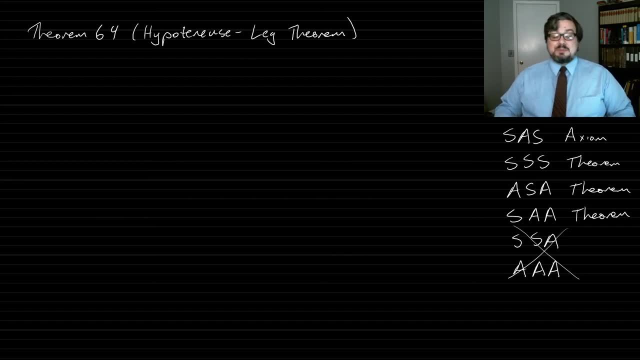 two sides and an angle that doesn't lie between them is enough in order to show that the triangles are congruent. So theorem 64 says that, given triangle ABC and triangle DEF, if angle A and angle D are right, then the triangle DEF is right, And if angle A and angle D are right, 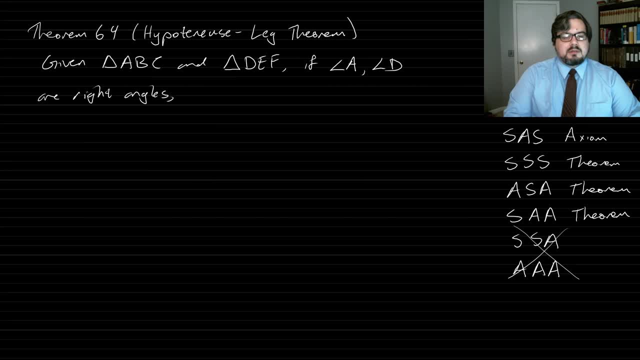 then triangle AB is congruent to triangle DEF. And if triangle AB is congruent to triangle DEF, then triangle ABC is congruent to triangle DEF. So the picture for this is that we've got a couple of right triangles- hence the name- hypotenuse, leg theorem. We've got A, B, C, D, E, F, And we are told that both the angle at A and 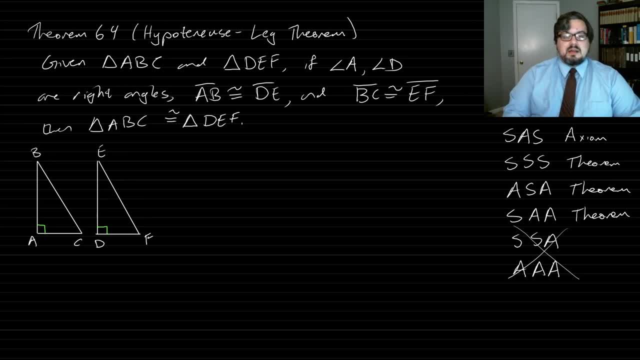 the angle at D are right angles, hence, of course, they're congruent. We're told that A, B is congruent to D, E and A C is congruent to E- F And, as I said, this is a side-side angle type of situation which is normally not good enough. 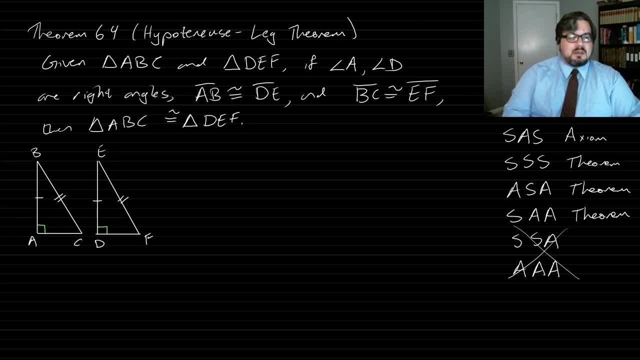 but in this case we can work with it. In particular, as is common, we're going to copy one of the triangles onto the other. So what we're going to do is we're going to basically copy D, E and A, C, And we're going to copy one of the triangles onto the other. So what we're going to do is we're going to basically copy D, E, F. 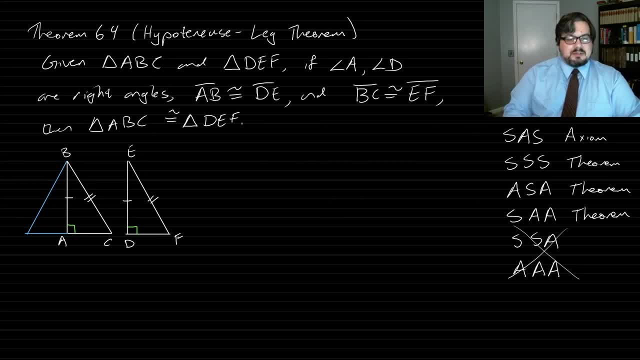 So what we're going to do is we're going to copy D E F, or a copy of D E F, onto the other side. Pardon me, We'll put D prime over here, So let's let D prime. 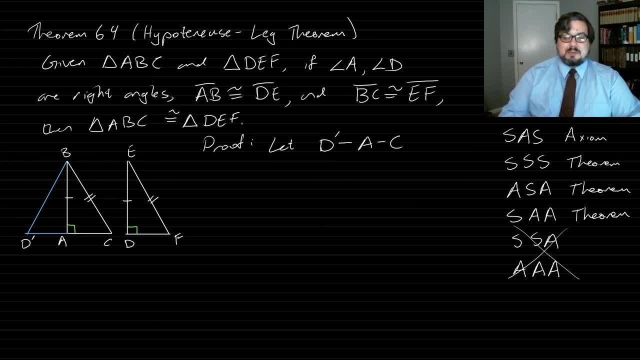 lie between— or let A lie between- D, prime and C, such that the segment D prime A is topping out. so A is approximately P plus D, which is more, if we're going to say, if we're going to put D, F on it. 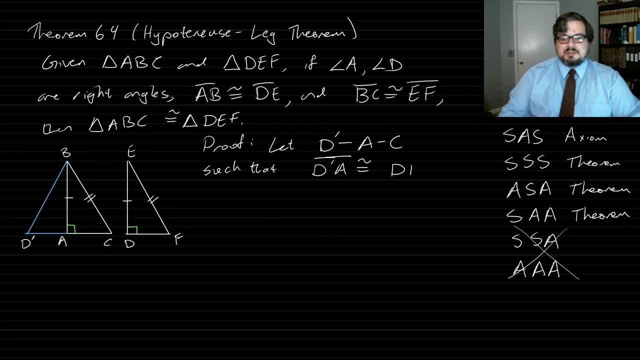 D, F on it— A is congruent to DF. Now we have that angle, BAD prime is a right angle because it's the, it forms a linear pair with a right angle. so in particular, this means that triangle BAD prime is congruent to triangle EDF by side- angle side- because 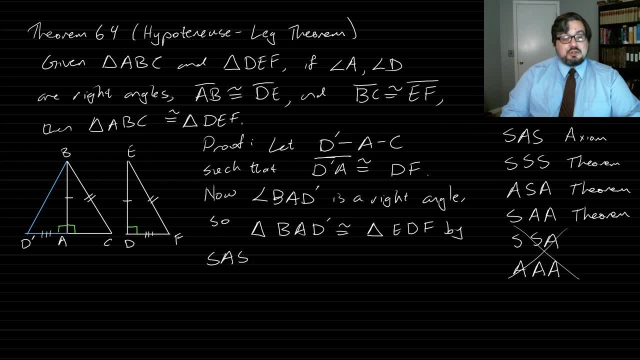 they share their congruence on the sides with two, with one mark, and with two marks, I'm sorry, and with three marks, and so that means that we've got the segment BD is congruent. so that means that the segment or BD prime, rather segment, BD prime- is congruent to segment. 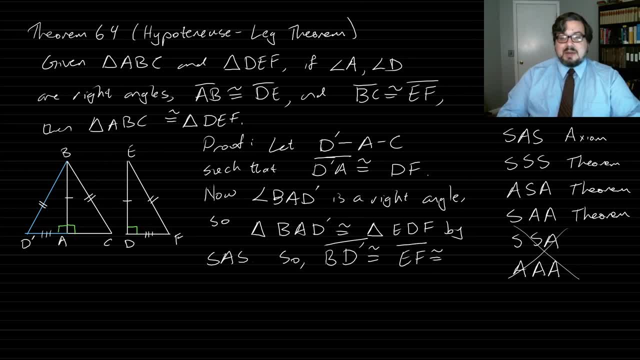 EF, which itself is congruent by hypothesis to segment BC. so that means that triangle BCD prime is isosceles. hence the angle at C is congruent to the angle at D prime, which of course is congruent to the angle at at F. I really should have used F prime instead of D. 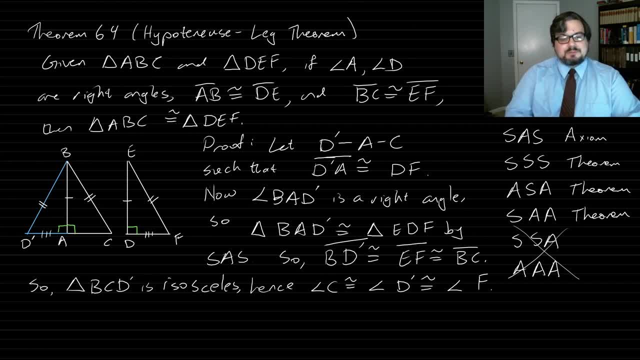 prime. sorry about that, but it still works. it's just not as elegant as I would like. so we have that. all of the red angles are now congruent. the angle at C and the angle at D, prime are congruent because they are angles in an isosceles triangle- opposite congruence. 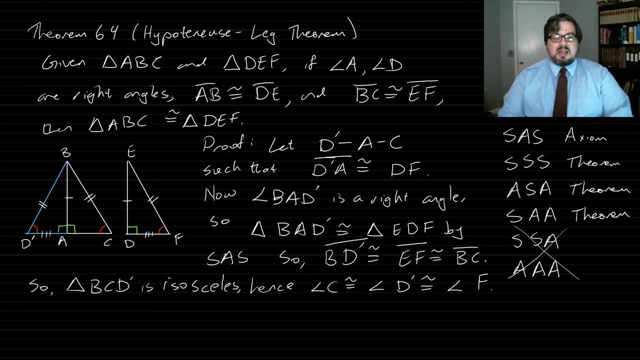 sides and the angle at D prime is congruent to the angle at F because the angles BAD prime and EDF are congruent. so now, if we compare ABC and DF, we have two angles congruent and more than one pair of sides congruent. So by angle,